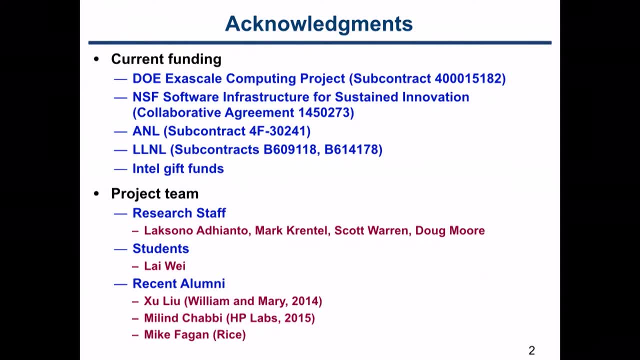 We had no idea why the codes were slow, and so instead we used compiler technology to build better tools to understand that, And so it initially started as something that was just an add on to our own research, and then it became a research focus in its own light as things got more interesting and the 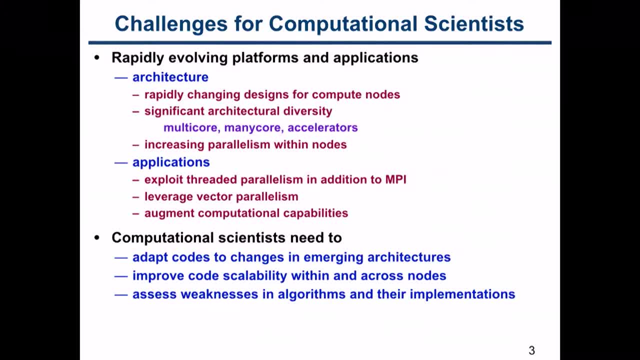 architectures kept getting increasingly complex. So some of the challenges for you, you as computational scientists, as I'm sure you're aware, after today. Personally, I was going to say the architectures are changing at breakneck pace, but hey, we're still computing in silicon. 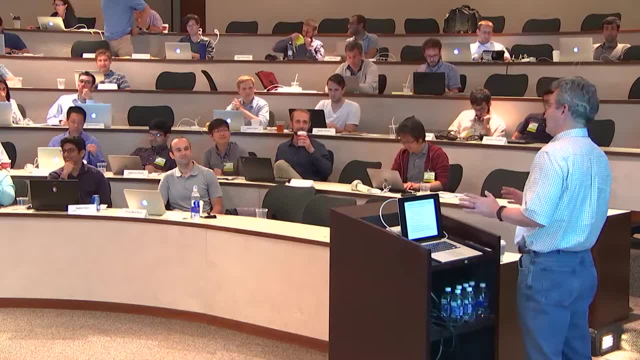 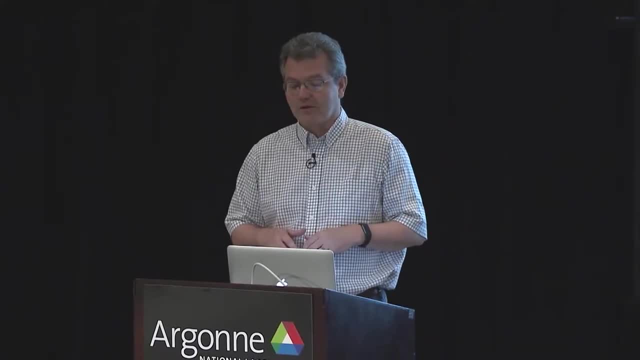 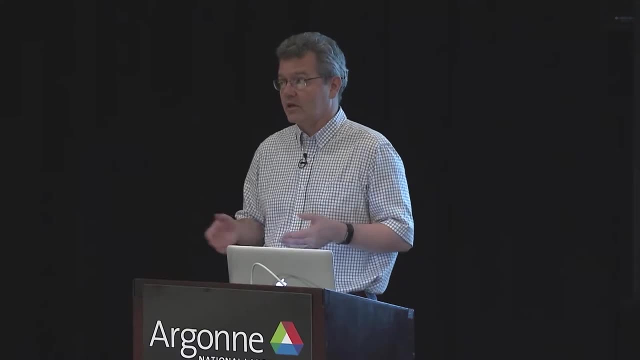 So now I feel better about what we're doing. So there have been rapidly changing designs for the compute nodes and there's a significant architectural diversity. So we have multi-core processors that are common in clusters. We have many core processors, like the Knight's Landing that you have in Theta, and 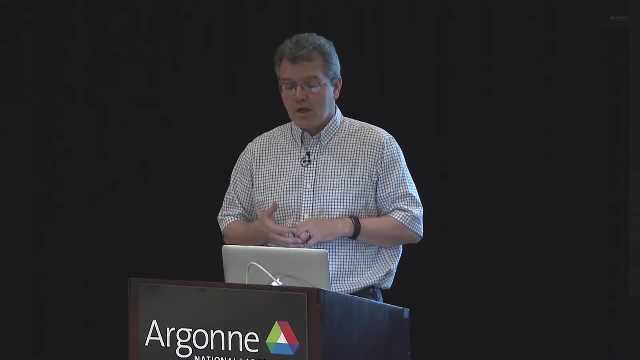 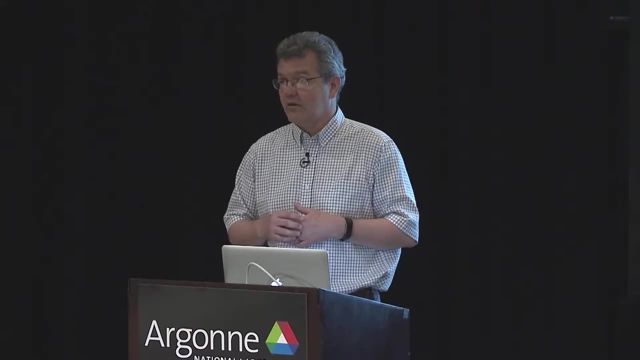 some of the machines at other supercomputer centers around the country, And then we also have graphics processing units as accelerators, And so the next generation systems that are coming out at Oak Ridge and at Lawrence Livermore are gonna be power nine systems accelerated with NVIDIA GPUs. 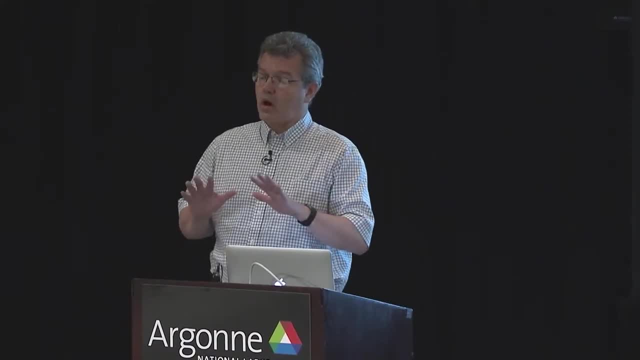 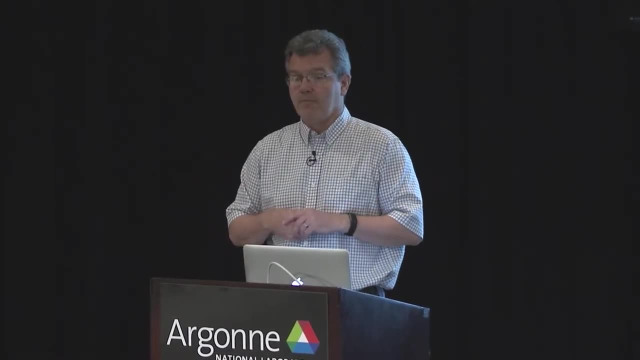 So while I don't envy you for you folks trying to develop applications that might run on one architecture and then run on another architecture, well, I have to tell you that from the tool side, it's even harder, because we don't get the luxury of all these levels of abstraction. 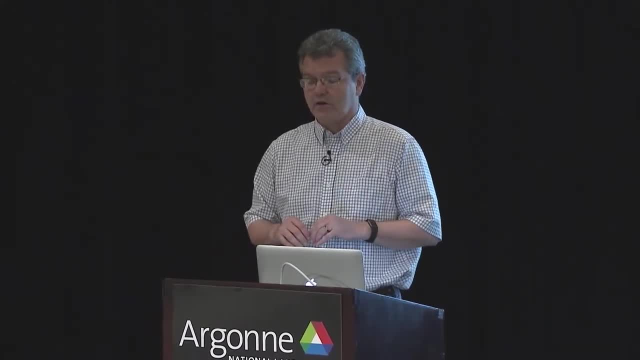 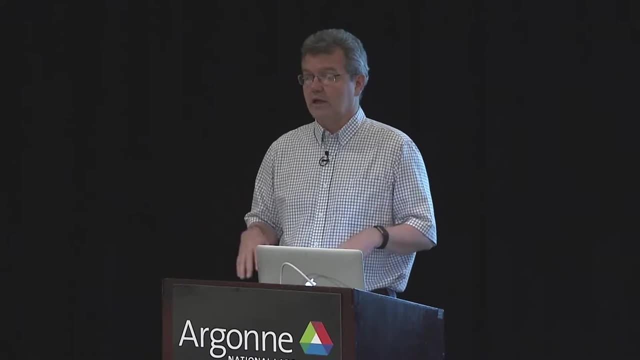 We have to know everything of what's going on down at the architecture level and at the OS level as well, and the OSs are not all the same. Well, today things mostly look like Linux, but on Blue Gene Q that's really not the case. 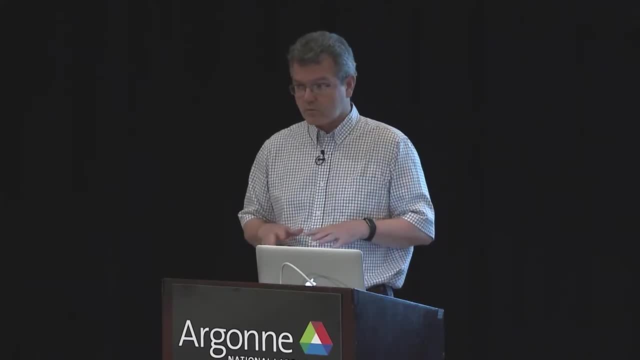 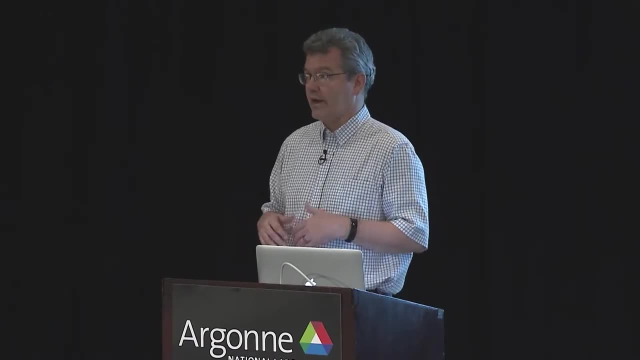 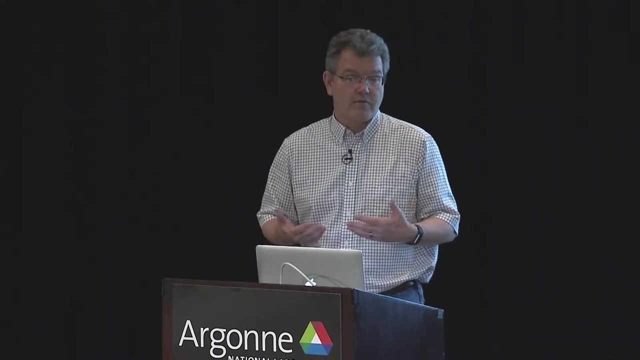 So there's significant architectural diversity. there's significant diversity in the software. There's increasing parallelism in the nodes and for the applications. what this means is that people need to be adding more parallelism to their applications if they're gonna get benefit of any of the micro architectural improvements. 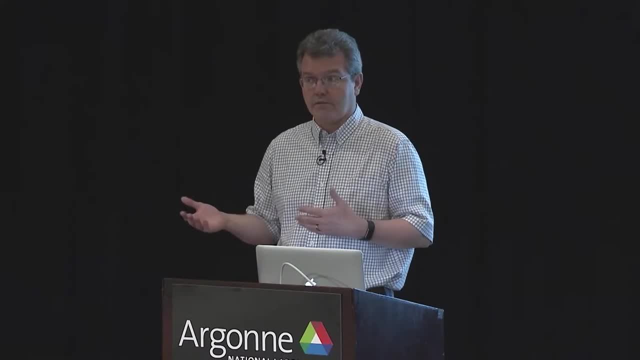 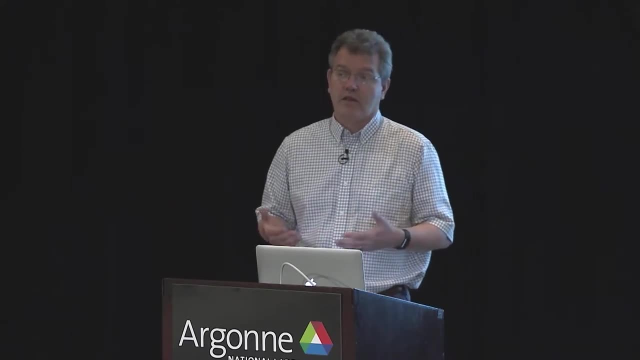 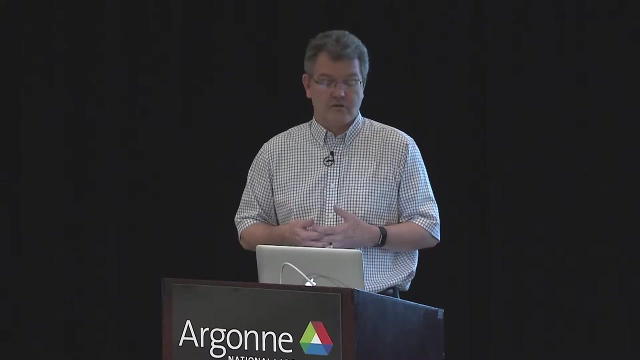 So you need to exploit threaded parallelism in addition to MPI. on typical architectures There's large scale data parallelism, either in the form of vectors on the Knight's landing chips Or the SIMT parallelism that you see- the single instruction, multiple threads that you see on GPUs. 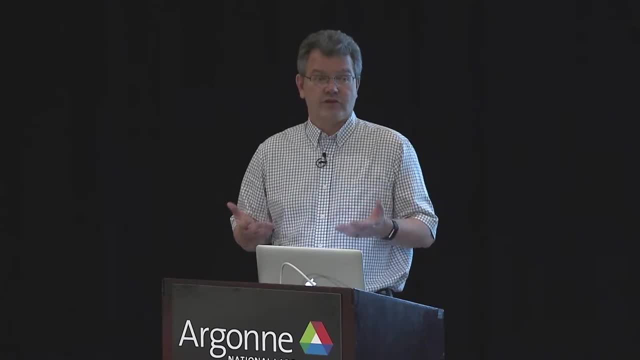 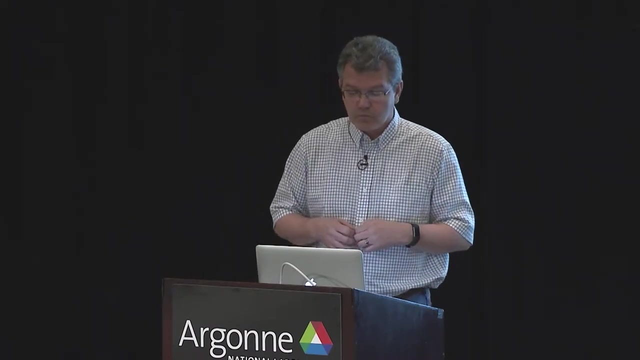 And so there's a lot of changes to just adapt the applications to deal with this influx of parallelism, as well as to augment the computational capabilities, because I'm sure that everybody would like to be solving a higher fidelity problem than their solution currently admits. 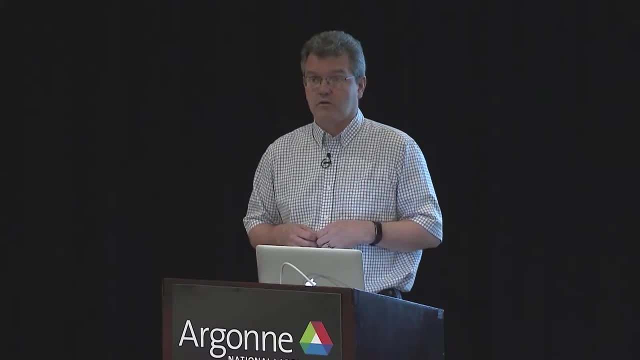 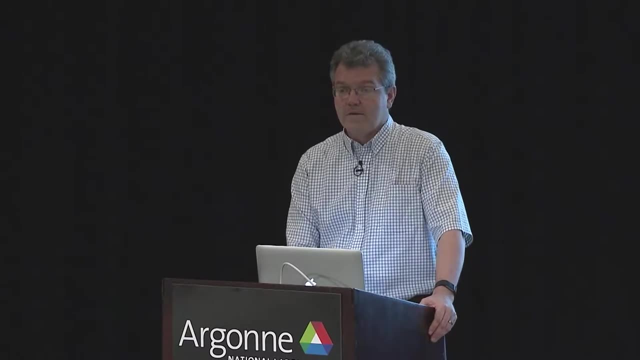 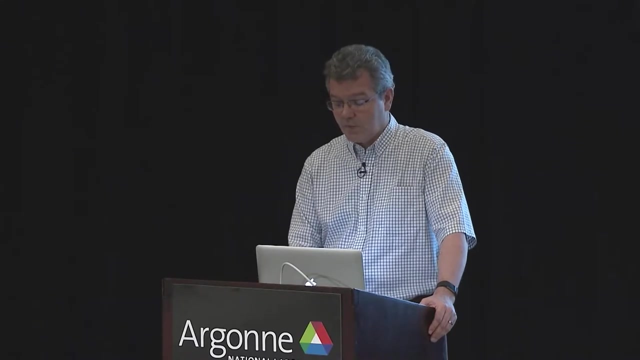 So, as computational scientists, you need to adapt your codes to adapt to the changes in architecture, improve the scalability across the nodes and assess weaknesses in your implementations And figure out how to invest your effort wisely, And so my contention is that performance tools can help play. 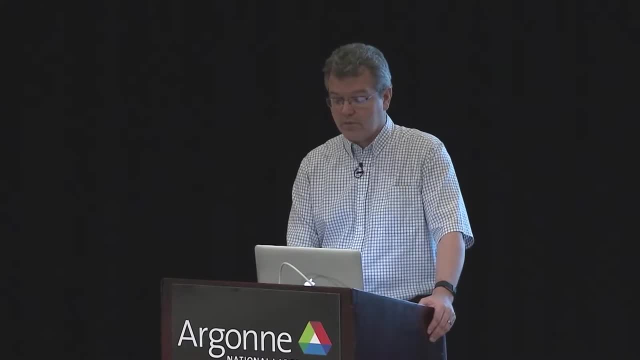 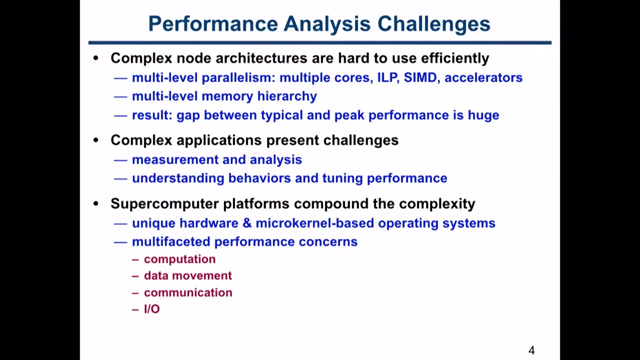 an important role as a guide as you invest your effort on your codes. So some of the challenges that make these systems so hard to use efficiently: you have complex node architecture. You have multiple levels of parallelism, So you have multiple cores, instruction-level parallelism, SIMD parallelism. 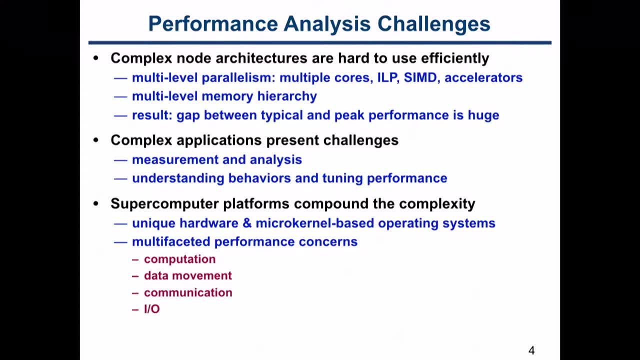 or short vectors. You have accelerators with a single instruction, multiple thread, parallelism. We have a multi-level memory hierarchy, So the memory- not all loads- are delivered in the same latency. In fact some of them are delivered very quickly. 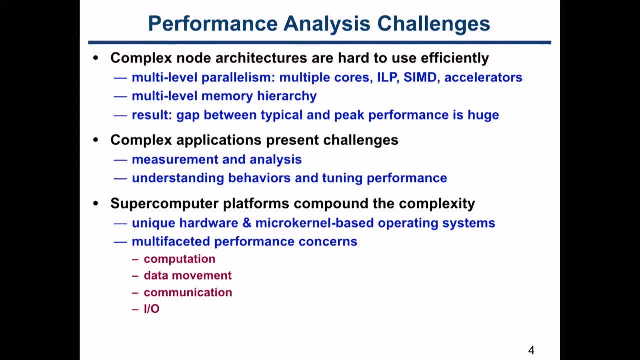 If they're in cache, that's close to the processors, But if you have to go all the way to main memory, it's a couple hundred cycles, And so, as a result of this complexity, the gap between typical and peak performance is huge. 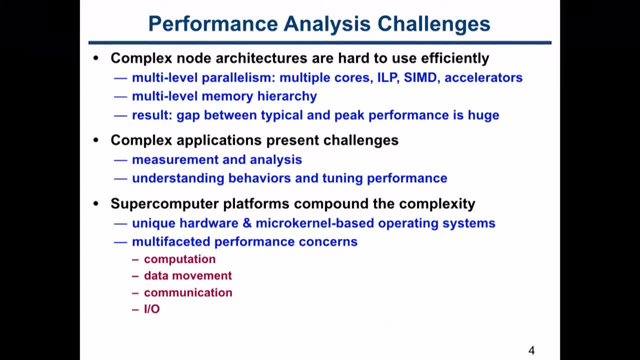 And so you really need performance tools to try and understand where there's sort of soft targets where just a little change in your application can give you maybe an integer factor of performance improvement which means that you're going to be able to get more out of your allocation on one of these systems. 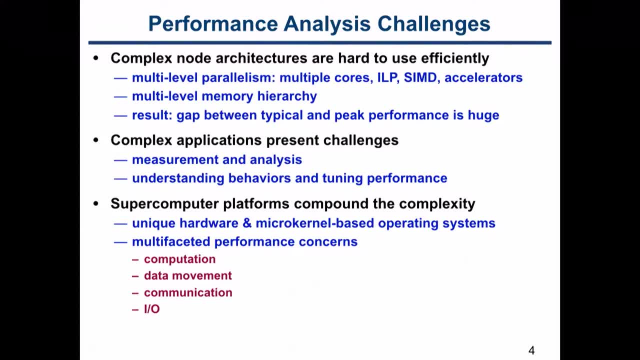 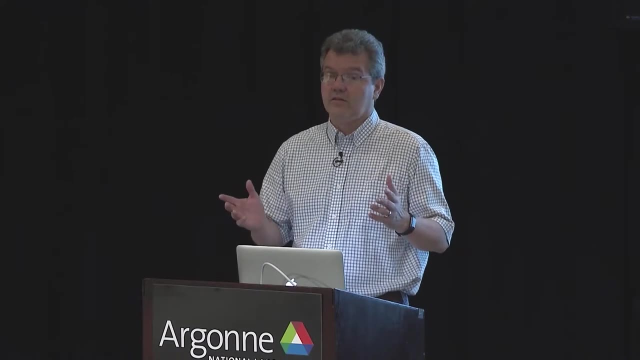 if you can solve larger problems or solve them faster and be able to run larger ensembles, for instance. So complex applications present some challenges for both measurement and for analysis, And understanding the behaviors and tuning the performance is very difficult as well, And it's not just a matter of if we know where the performance losses are, then it's easy. 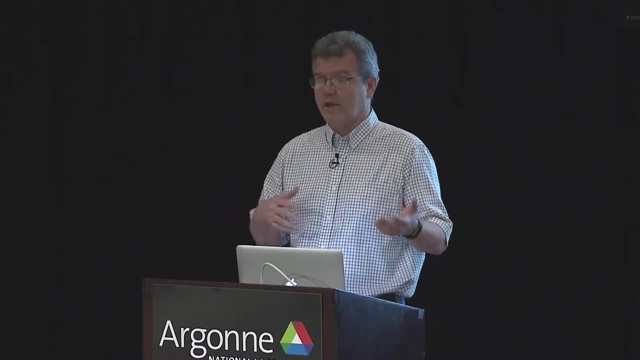 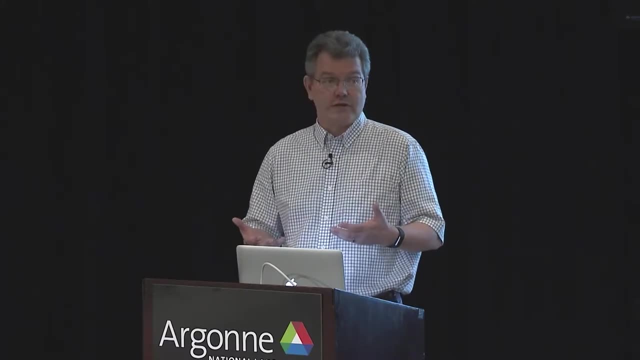 because sometimes it means changing all of your data structures and changing the way that you divide up your computation and whatnot, And so I think just getting the data is really sort of the first part of the journey towards fixing your application and tailoring them for better scaling. 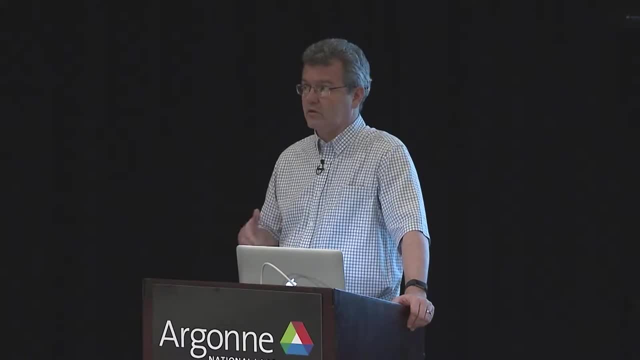 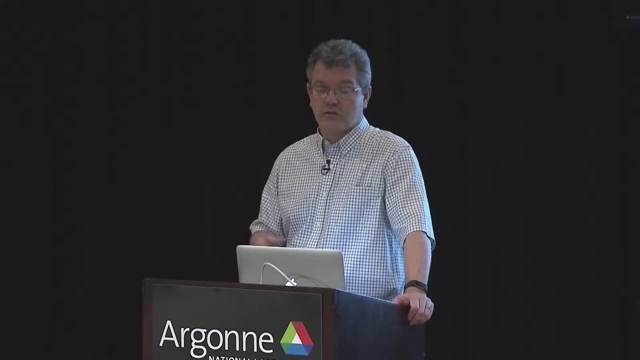 And on supercomputers, we don't care just about the performance of the compute engines, we also compare about, we care about the data movement costs, we care about the communication, we care about the IO, And these are not solved problems. because if you want to know, 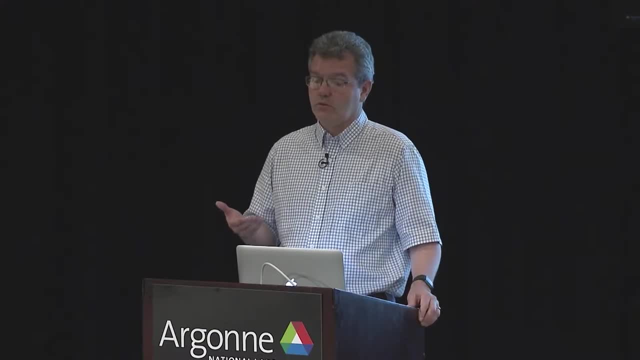 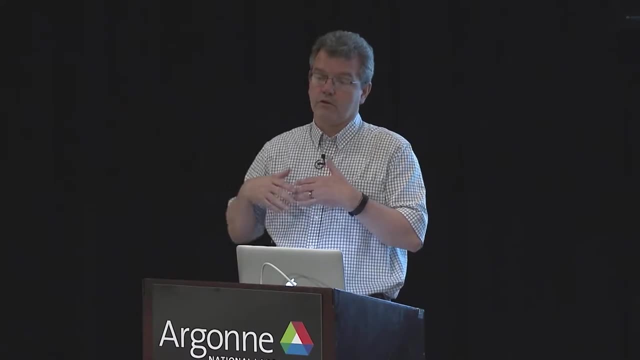 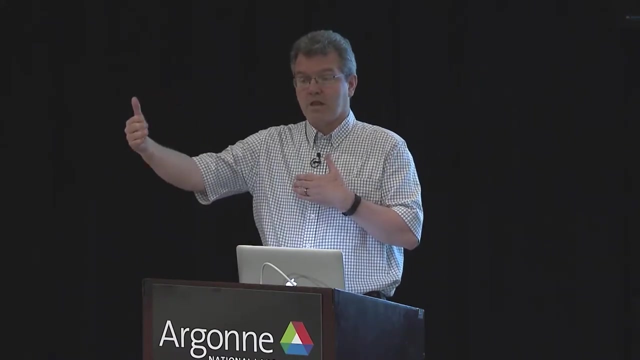 the reason why your IO performance isn't what you're hoping. this may be very, very far from the processor where your measurement capabilities are, And there may be contention for shared disks. there may be a cable that has intermittent failures. you may be conflicting with other jobs. 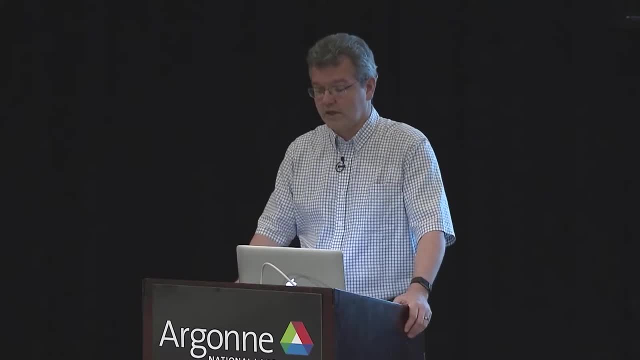 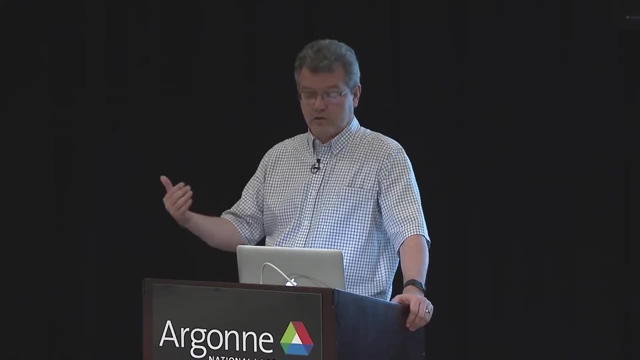 there's all sorts of things going on in the system and it's hard to measure things these days, And so one of the things that we're doing as a community is trying to work with the vendors and try and get some more measurement interfaces in the networks and IO. 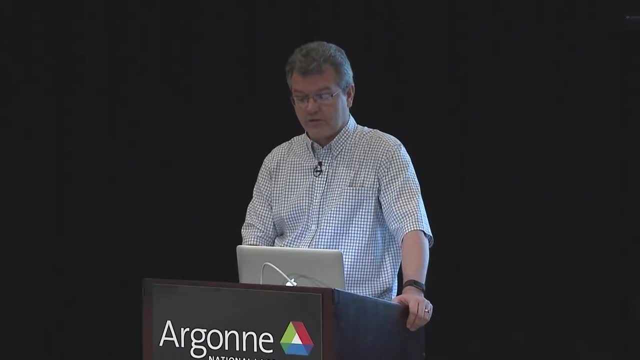 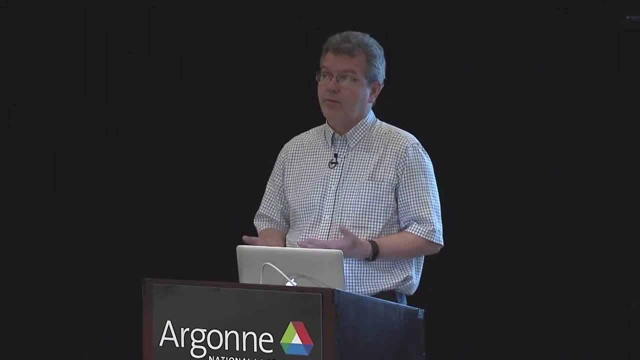 which isn't going to solve the problem for today, but maybe next generation or the generation after that, And that will be a little bit easier. So what I would argue that users want is multi-platform programming model, independent tools, whether you're writing an MPI or whether you're using 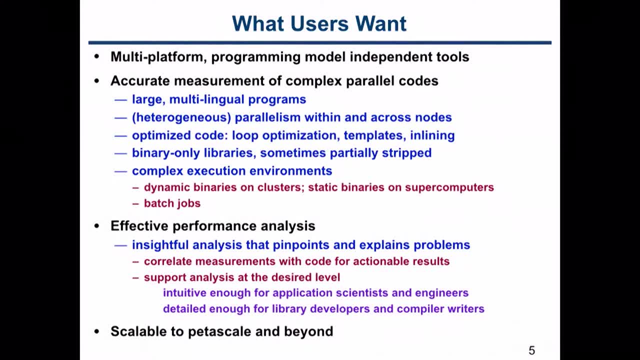 a partition global address space language, like a shared memory computing model on clusters and supercomputers. you'd like to be able to use the same set of tools. You'd like to have accurate measurement of parallel codes. the codes might be multilingual. 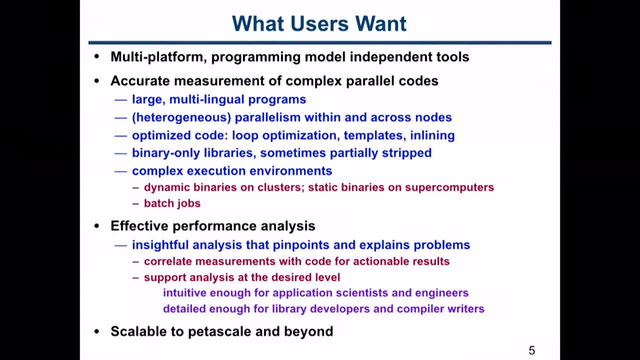 parts of them might be in C++, using templates. you might have some kernels that are written in Fortran, or libraries that are written in assembly code, or they're in stripped code, as is often the case. NVIDIA strips their libraries. that's part of their release process. 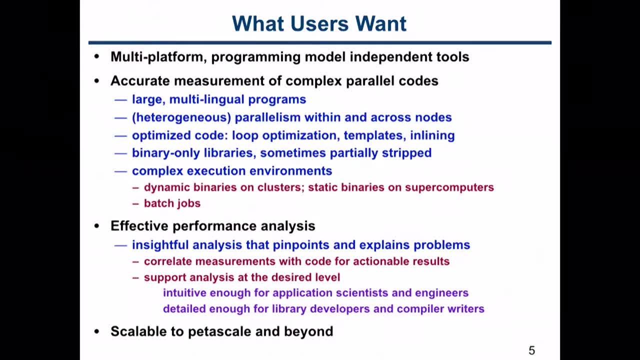 and so do some of the other software vendors, And so we have to be able to deal with code that's been optimized in many ways: loop optimization, template instantiation and inlining binary only libraries, complex execution environments, So on clusters, when you launch a program, 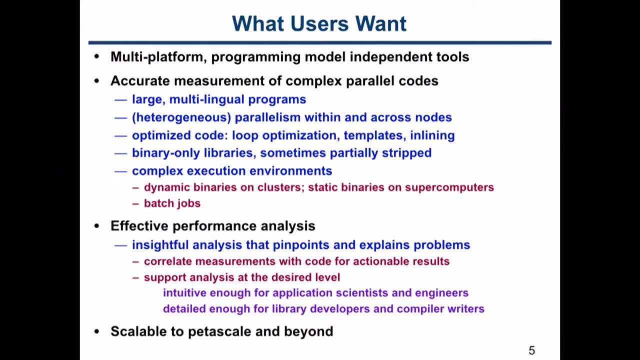 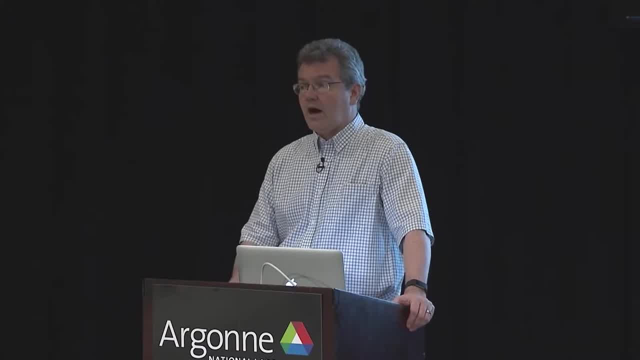 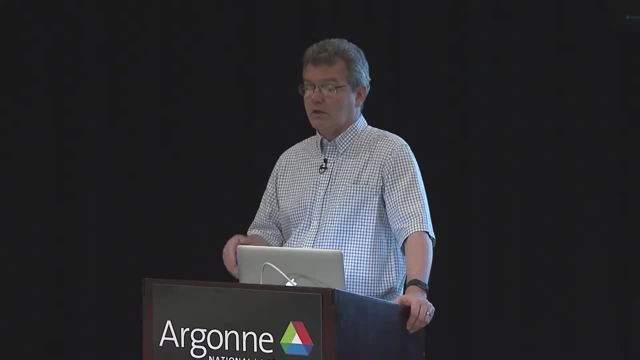 there are all these libraries that it refers to that aren't actually linked as part of your program, and so code gets dynamically loaded into the address space of an application as it executes. On systems like the ones at ALCF, typically the applications are statically linked. 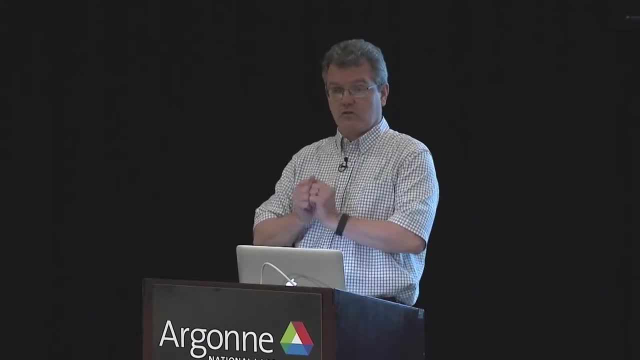 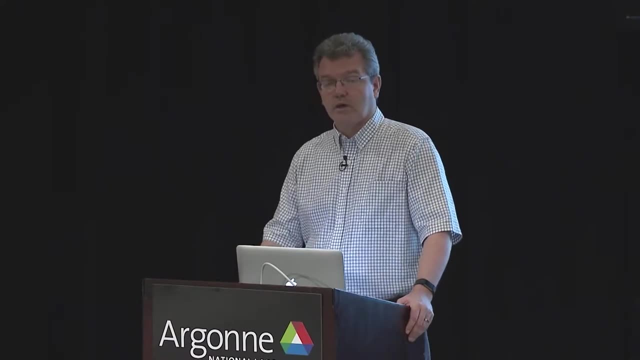 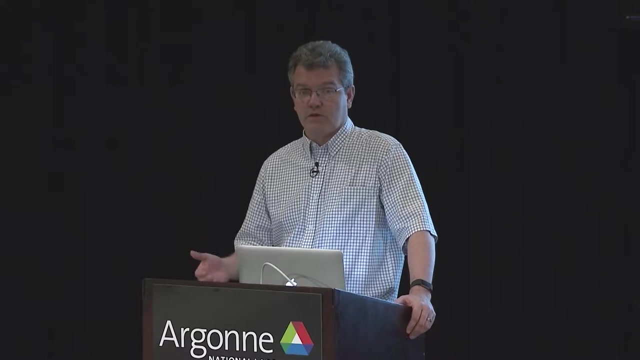 so that all the code is part of the application, because that makes it easier to just distribute to the compute nodes and know that you don't have to go back for anything more. However, that's also changing as well, because the next generation Coral systems with the IBM power systems plus the NVIDIA GPUs. 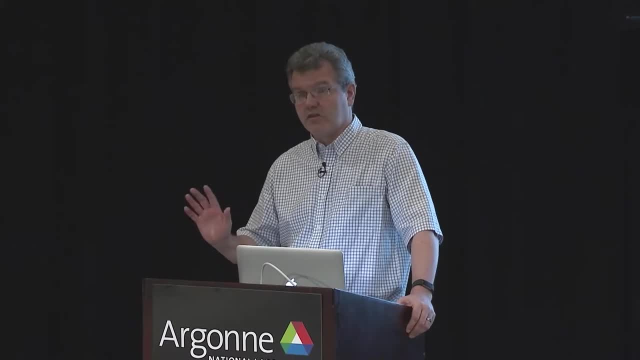 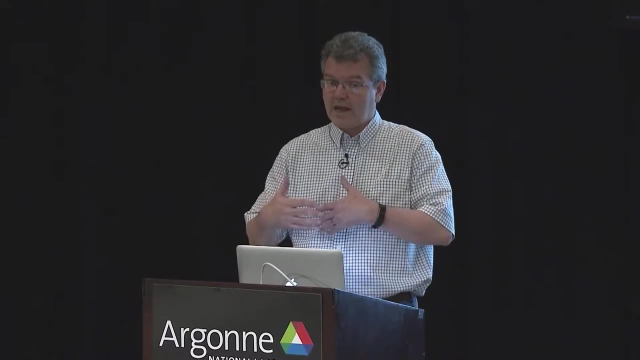 they're expecting to use those dynamically linked, and so they have to make some accommodations for that. So the point is that the environment that we have to measure applications. sometimes we have all of the code as part of the application, other times there's code. 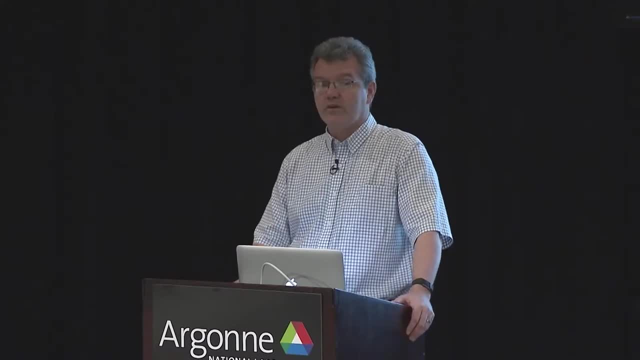 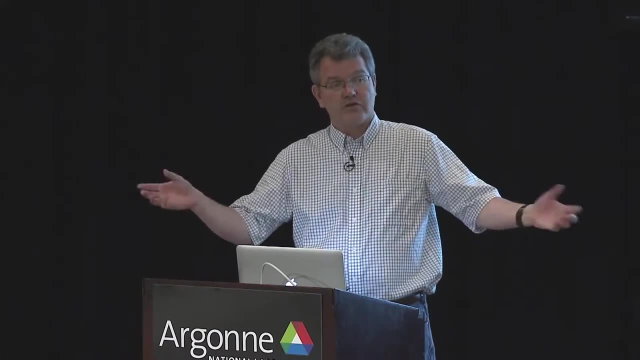 that's just appearing into the address space and we need to measure it all, And so we can't just add instrumentation to your application. We need to measure instrumentation as it gets compiled, because there's all these other pieces of things that you're using: the math library and libc and whatnot. 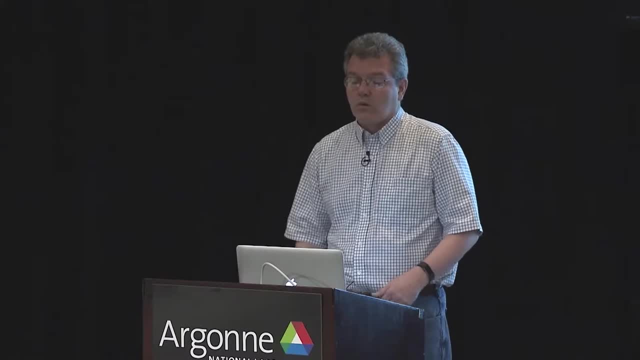 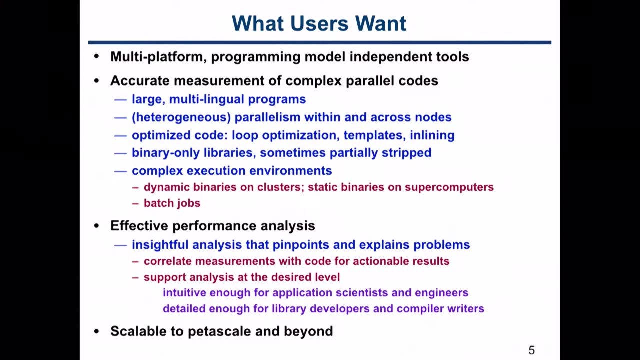 which don't have instrumentation embedded in them. So what I would argue, you want is some effective performance analysis that pinpoints the problems and then also gives you some insight into what the nature of these problems are, and it should be accessible at a high enough level. 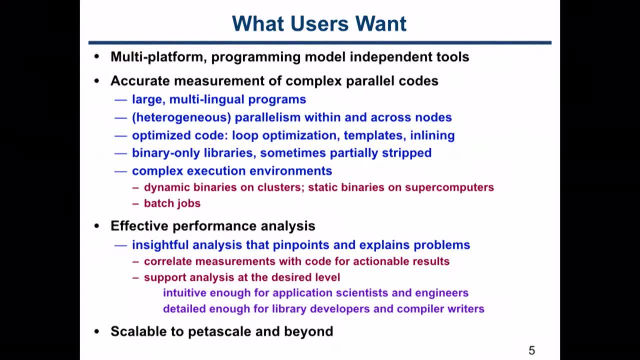 that a casual computational scientist should be able to figure out what the major performance problems are in the program. but also we are trying to build tools that would let compiler writers and library writers eke out the last bits of optimization. So we want very detailed information and then just reveal it. 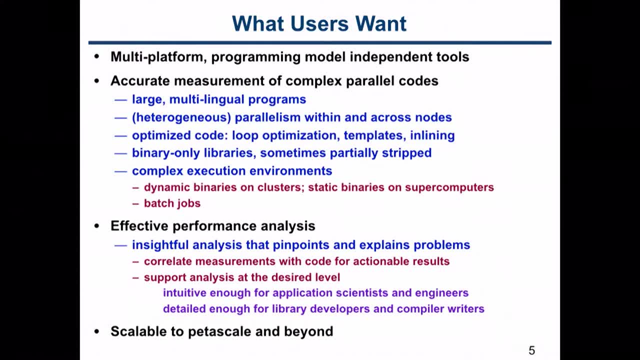 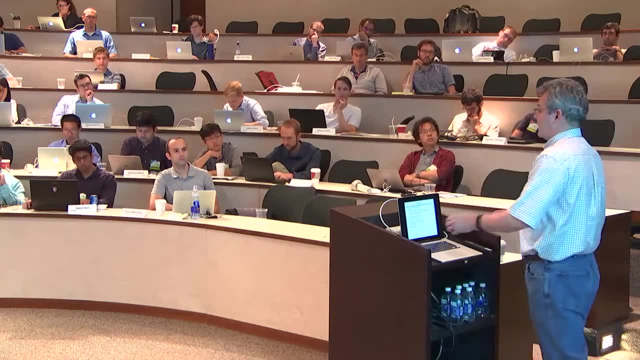 in sort of a level by level fashion, And we don't like this all to scale to large scale systems. So let me tell you a little bit about Rice University's HPC toolkit, Which is available on the ALCF systems and other centers around the country. 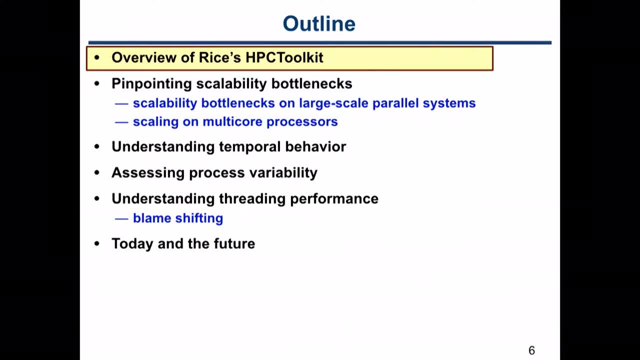 and also around the world as well, And then I'll show you how we can use this to pinpoint scalability bottlenecks and how we can use it to understand application behavior over time, assess the variability across processes and threads. a bit about understanding threading performance. 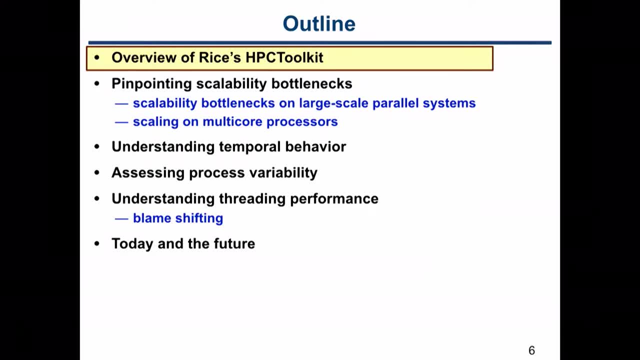 because threaded programs, OpenMP threading or other kinds of of multi-threading using either the Raja portability layer at a template based programming model at Lawrence Livermore or the Cocos template based model, Vados Sandia- There's a lot of different ways that people are looking at exploiting threads. 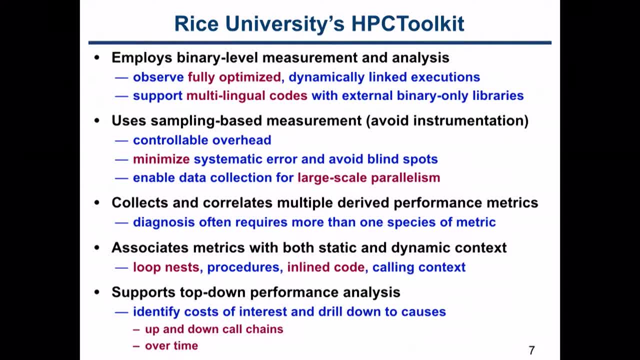 So I'll start by telling you a little bit about what HPC toolkit does. So it employs binary level measurement and analysis. What we're doing is we're observing fully optimized executions. So if there's loop optimization template inlining, we want all of that in your code. 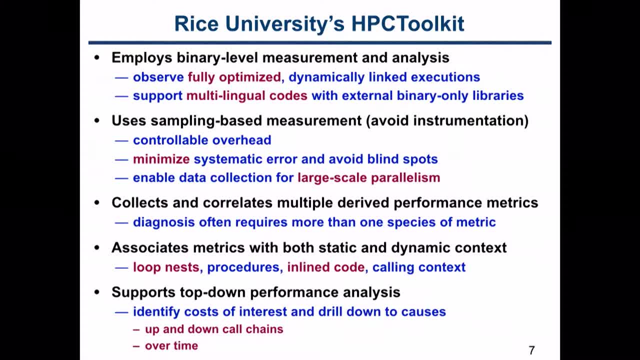 We don't want to say you can only analyze and understand performance of unoptimized code. The strategy that we use for measuring an application is we use sampling, And so we typically avoid instrumentation. There's a little bit of instrumentation in the program so that we know that when threads are getting created. 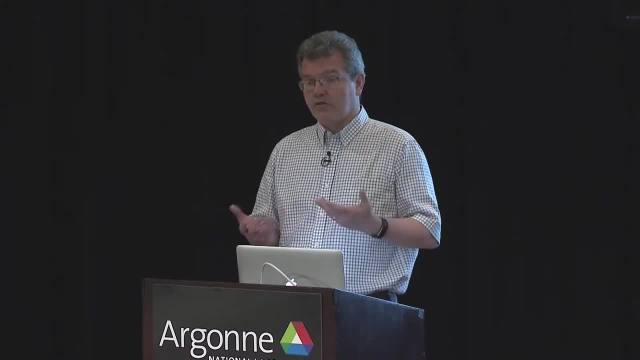 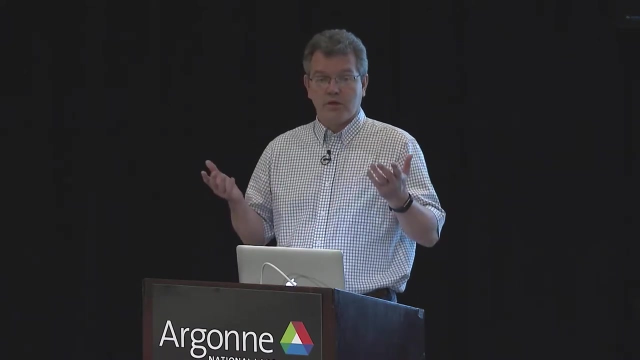 or when threads die or things like that. But generally we are periodically interrupting the program to find out what's going on. So we might interrupt based on time or we might set up certain hardware performance counters so that they will periodically signal us like every million cache misses. 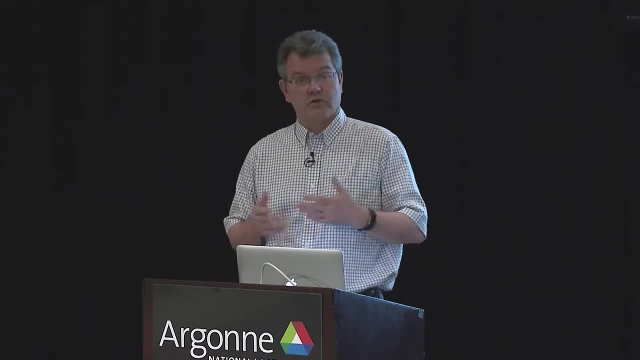 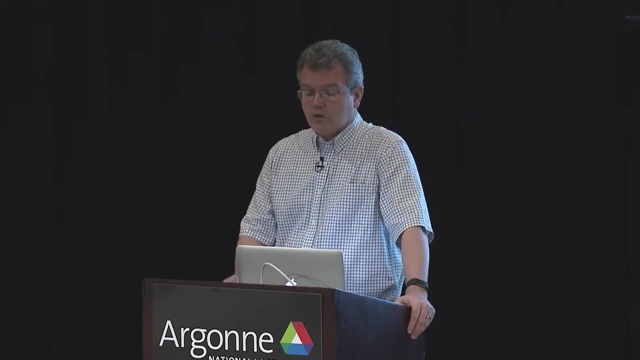 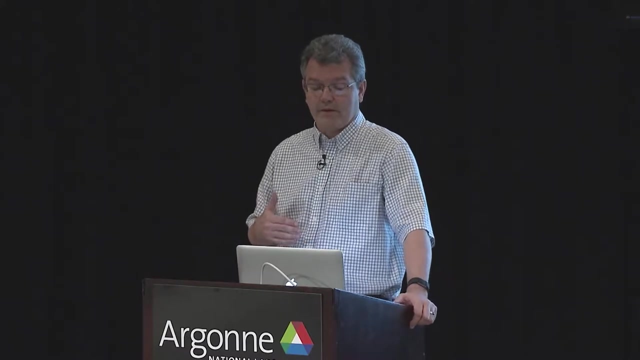 or every so many translation look-aside, buffer misses or things like that, So we can keep track of what's going on in the memory hierarchy and know when data is moving. So the sampling-based methodology enables us to have low, controllable overhead and also the amount of data that we collect. 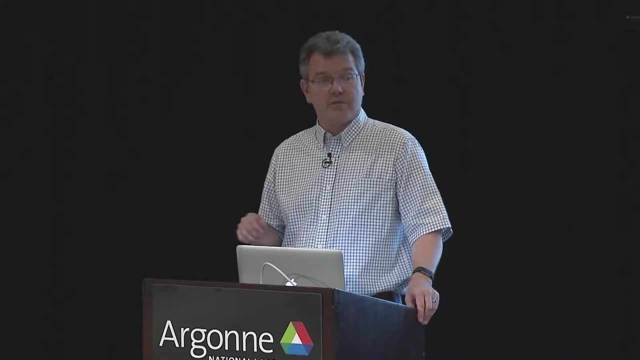 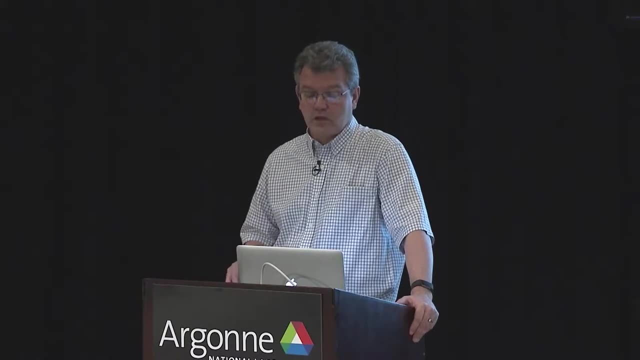 is relatively modest. We can scale down the amount of data by just turning down the sampling frequency, And so what typically is useful is to collect and correlate multiple kinds of performance measures, And so if someone says well is a billion cache misses a lot. Well, it depends. I mean, if you're doing trillions of instructions, then a billion cache misses might not be a big deal, But if you're only doing on the order of a billion instructions, then a billion cache misses is a lot. 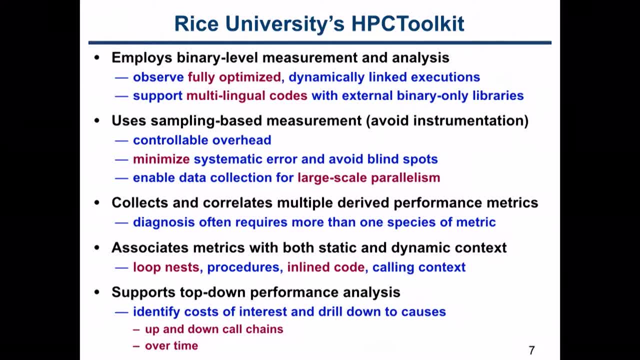 So you often need multiple metrics in order to put things in context and decide whether you have some performance problems. So our tools associate metrics with both static and dynamic context, So you get things associated with source lines, procedures, but also loop nests and inline code. 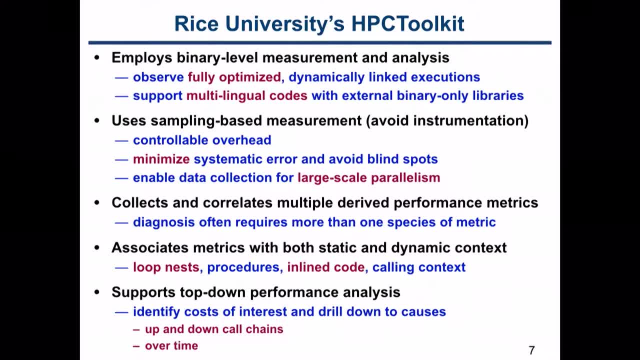 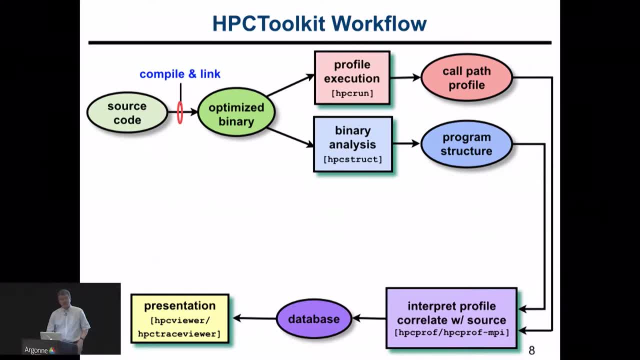 and entire call chains. And then a key feature of the way that we designed our tools is that they support top-down performance analysis. So when you use our tools, there's actually only a few pieces in the toolkit and there's a very uniform way for using them. 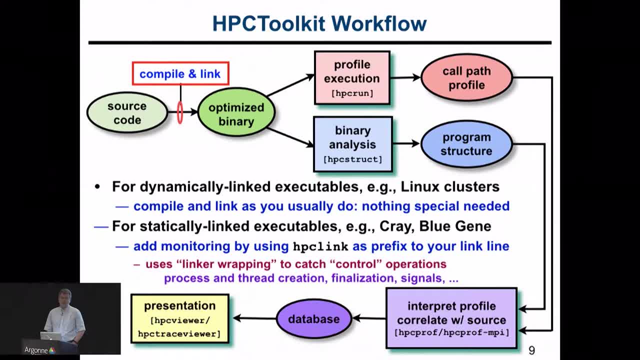 So you compile and link your programs the way that you normally would, And so, if you were using a Linux cluster with dynamically linked binaries, there's no changes until you just launch the tool with our launcher. However, when you're using these statically linked binaries, 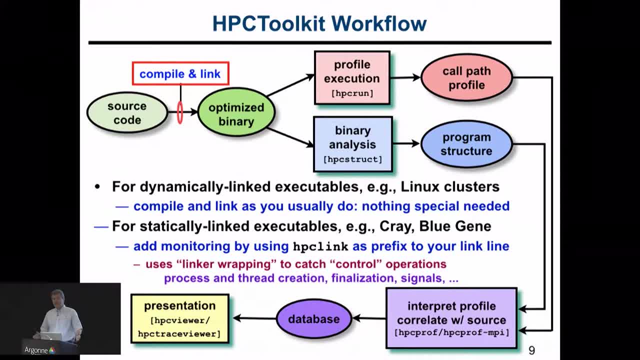 on the supercomputers at the labs, then we do need to just add our library to your application and we have a wrapper script so that when you link your application, whatever your link line is, you just put our script in front of it. 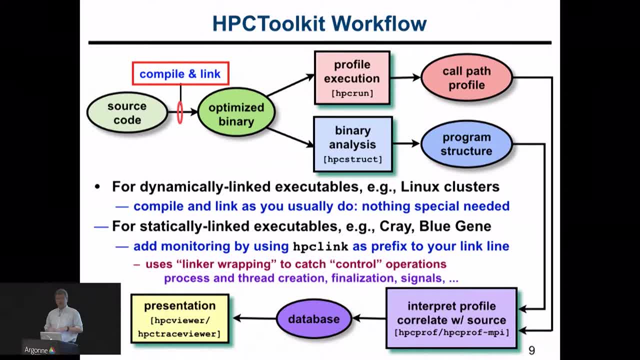 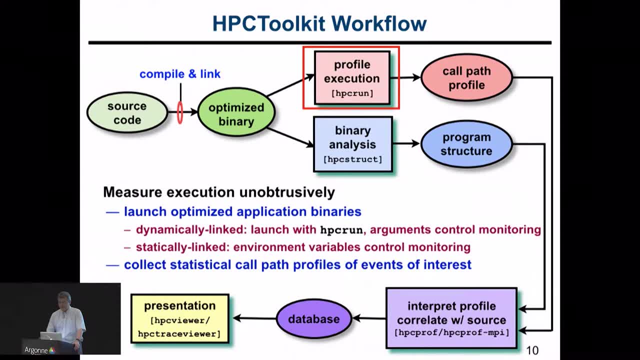 and it will do whatever it needs to do in order to get our stuff into your application. So there's really very little changes to the build process. And then, once you have your instrumented application- so it's either instrumented on launch by just dynamically loading code into the address space- 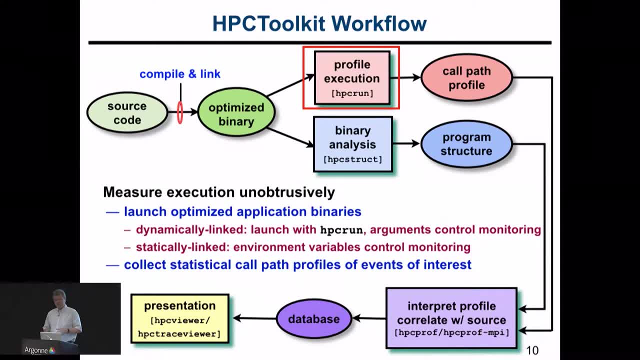 or we have our measurement library as part of the application. When you launch it, then you give it some arguments that say what you're interested in measuring or typically what you're interested in sampling. And when you're using our launcher, then you give it some arguments. 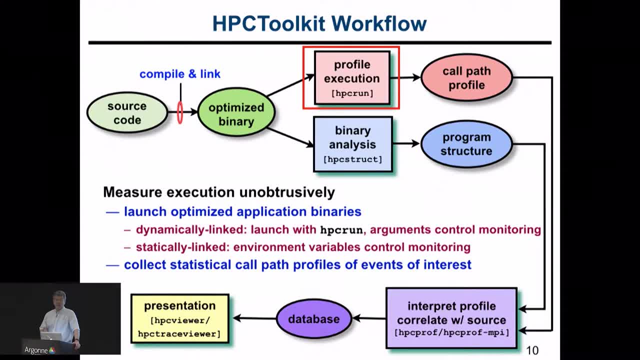 and then, as you launch your program, you say what you're interested in. Otherwise, if you've got statically linked binaries, then all the control is through some environment variables that you set as you launch the application, And what our tool does then is it collects statistical call path profiles. 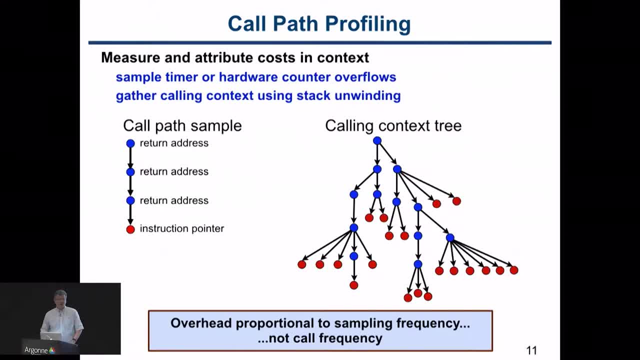 of events of interest. So what I mean by a call path profile is: at a particular point in time we get interrupted. Either a timer goes off or a threshold of a count of some kind of event in the hardware is exceeded, and we'll get interrupted at a particular instruction. 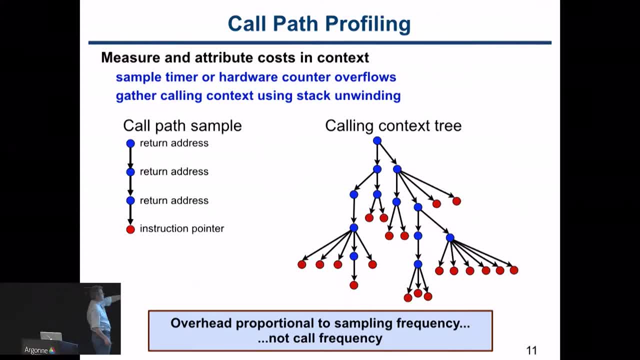 And so then what we want to know is okay. so maybe I'm in the middle of some routine C, when called from B, when called from A, when called from main. We want to know how we got there, okay, And so when we get one interrupt, 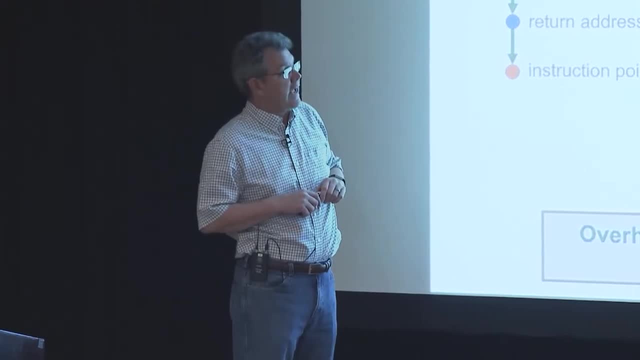 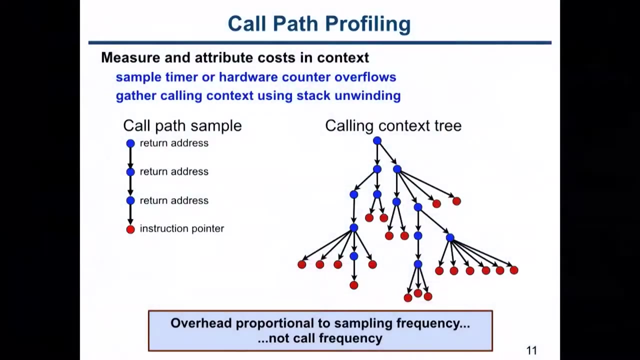 then we figure out what the whole call chain is And then over time, as the application executes, we accumulate a series of call chains and conceptually there's kind of main at the top and then some subtree might represent program initialization, some other subtree might represent a solve phase. 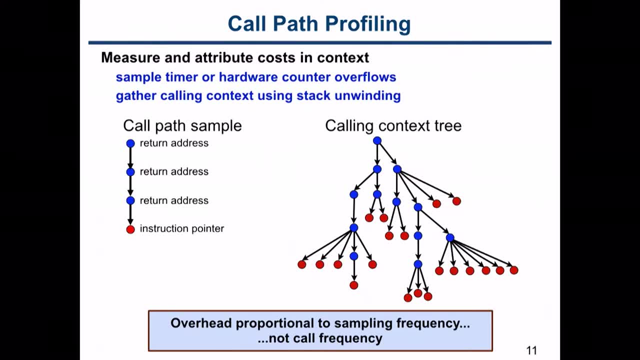 some other subtrees might represent post-processing or something like that. Now you might think that this is easy, but it's not So. actually we're doing dynamic binary analysis on the fly to figure out how to unwind the call stack of optimized code. 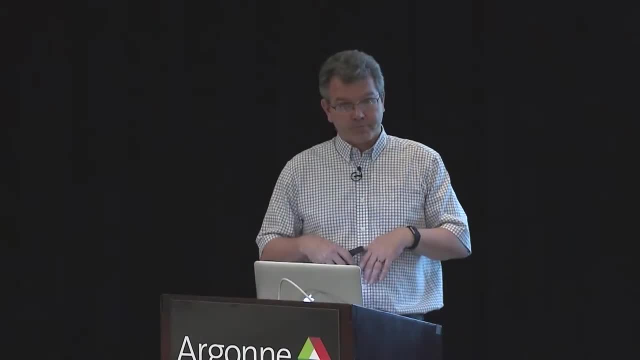 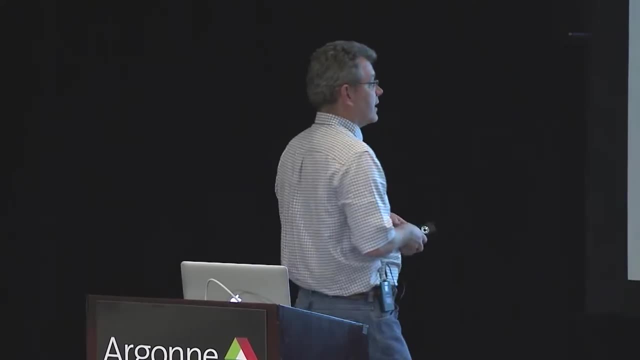 and caching our results. So, as your program's running, we're analyzing this machine code, and we're doing all of this with just a couple of percent overhead, And so the important thing for this sampling-based approach is that the overhead is proportional to the sampling frequency. 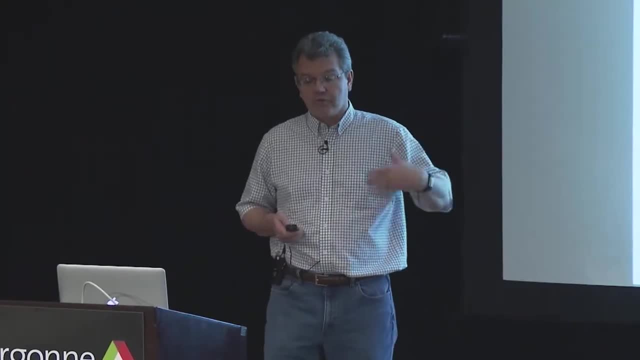 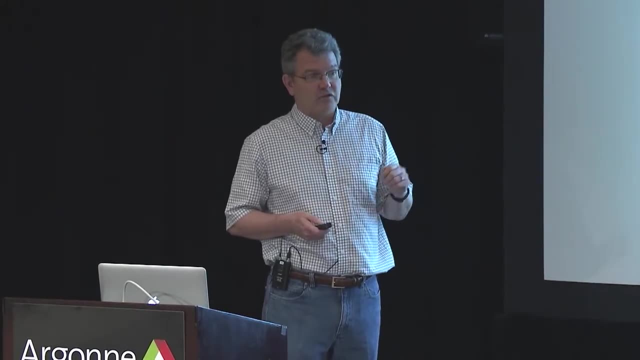 not the calling frequency. So it doesn't matter how frequently you're calling functions. You might have really tiny functions in your program Instead, if you just say I want to sample 1,000 times a second, then 1,000 times a second we get interrupted. 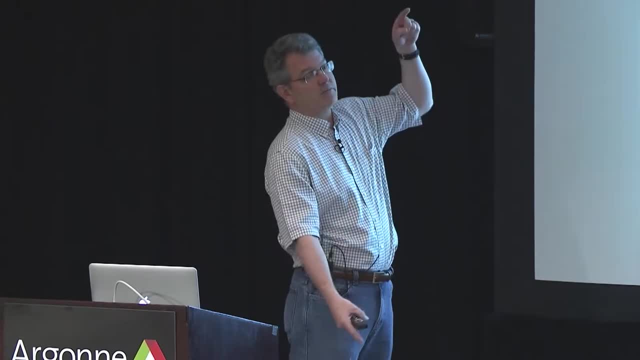 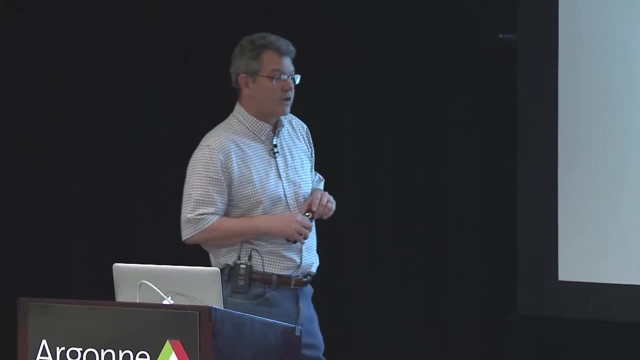 and then we're going to unwind the call chain. So if you have really deep call chains, then the samples are going to cost a little more, but that's not typically the case. So then the next thing we do is: So, that's our process. 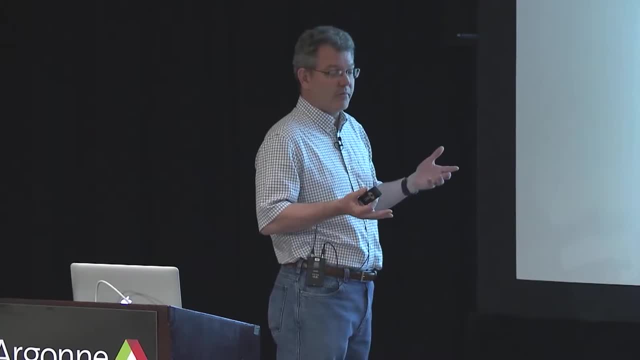 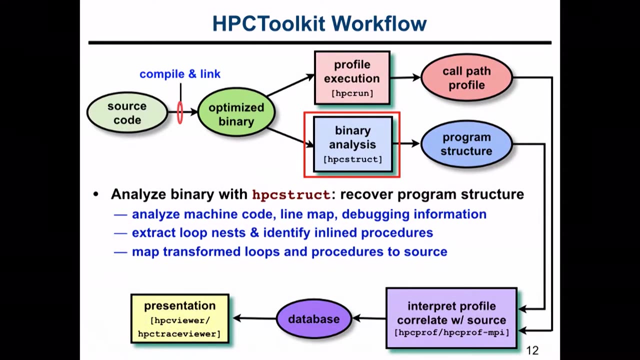 of collecting dynamic measurements about the application. We're collecting these call chains as the application executes. Then we do binary analysis to figure out how we're going to take all of these program counter locations and relate them back to your source code. So we analyze the machine code. 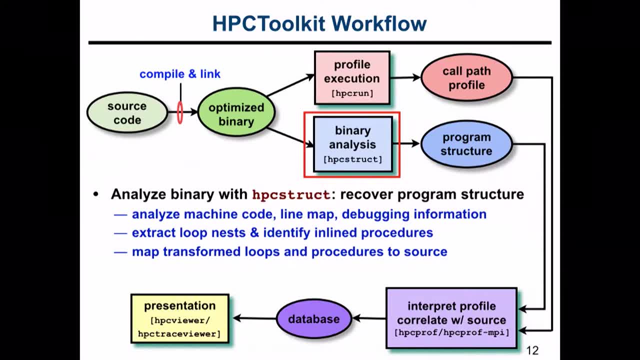 the line map, whatever debugging information the compiler may or may not have recorded, We extract loopness and identify inline procedures and we map all of the transformed procedures back to the source code. So there's this program analysis phase where we're trying to figure out. 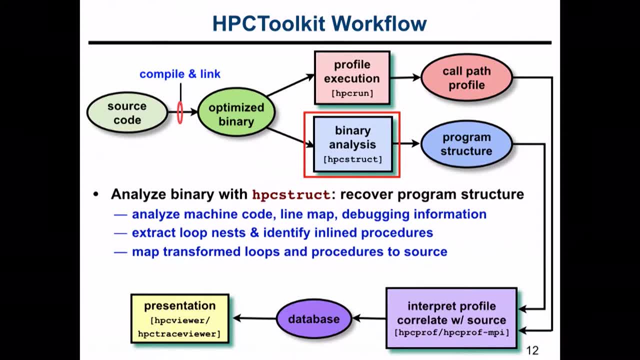 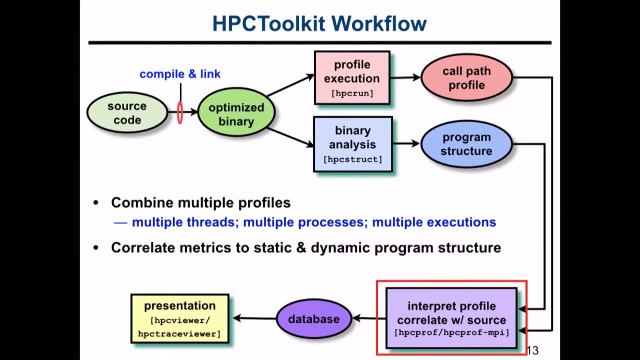 how all of the activity we observe relates back to your application. And then we combine. We combine the call path profile with dynamic measurements, with the binary analysis to interpret and correlate that with the source code. So you can combine profiles from multiple threads, multiple processes. 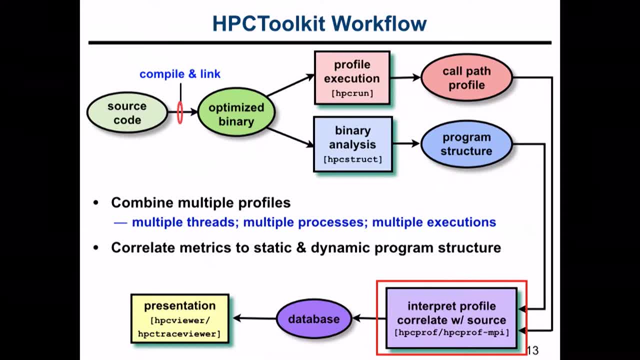 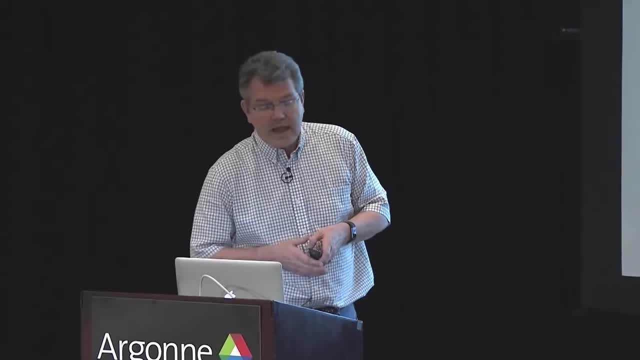 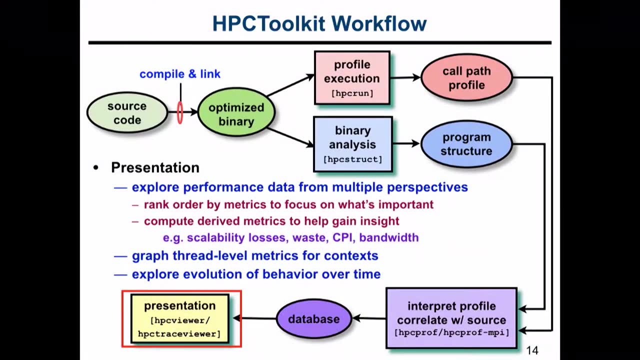 multiple executions and correlate them to both the static program structure, like loopness, and the dynamic program structure, like call chains. And then the last piece is: once we've computed all this information, then we have a couple of graphical user interfaces for viewing it. 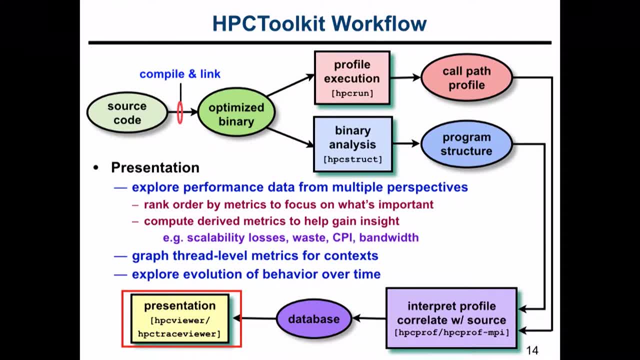 And so you can explore the performance data from multiple perspectives. You can rank order by what's important to you- not to us as the tool developers You decide. You can compute derived metrics like scalability, loss and waste and cycles per instruction and things like that. 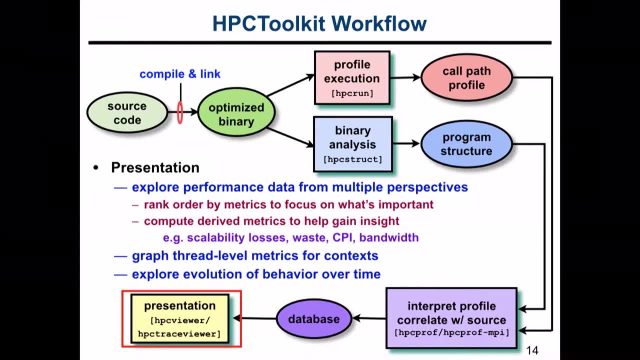 Whatever you think is going to give you the kind of insight. You can collect multiple sources of data and then combine them with equations to give you the kind of insight that you're looking for. You can graph thread-level metrics for context, and then you can explore the evolution. of behavior over time using these time-centric views. So here's our code-centric analysis and coming out in the user code in the Lambda functions on the other end. And so they use this to map code onto both GPUs and onto OpenMP as percent scalability loss. Okay, and I'll display this as a percent. Okay, and now I have an extra column and it says I've got a 24% scaling loss in scaling from 256K to 8K cores. And if I look at this, I can see that 14% of the scaling loss is in the evolve phase and 10% of the scaling loss is in the initialization phase. So I'm going to just select the column with scaling losses and then say, all right, so show me where the scaling losses are. So let me look in the initialization phase first And I dive down into the tree and say where the scaling losses occur. And so what this flame button does is it keeps opening Every time there's a child node in the tree. that accounts for 50% or more. of what I'm doing, then it just keeps digging down And so it's like trying to find the interesting stuff for you. You can set the threshold if you wanted, say 30% or something like that. So we end up down at this loop nest, okay. And now we look up a couple of lines and it says: loop through all processors. Well, as we go from 256 processors to 8K processors, we're going to go more trips around this loop. Okay, so that's. that's the root cause of our scaling loss. And you could ask: well, why are we doing that? Well, that's when things start to get complex. So it turns out that this loop has all of these send, receive, replace operations inside it. So what it's actually doing is: it's doing adaptive mesh refinement, You end up with some block that represents a part of the 3D domain and you need to know, after adaptation, who's got the neighboring blocks, And so this package had no idea or no knowledge of that. It just said: well, what I'll do is I'll package up the information about the blocks I have and I'll hand them to the processor on the right, and then we'll circulate these all the way around the ring and everybody will find out. what everybody else has, and then we'll figure out what we're doing. okay, And I'll like watch this stuff. go by and say, oh, I'm interested in that one. That's my front face, I'm interested in that one. That's my back face. So this cycles around a ring, And so that is the root cause of this scaling loss. And so Anshu Dube took a look at this data, and then they realized that because of the way they were using space-filling curves- in fact, they didn't actually have to ask everyone, They just had to kind of look in a neighborhood, And so pointing out this problem led them to change their algorithm and reduce the scalability losses. And so I'm kind of running short on time. but I can go and look at every percent and sort of drill down and find out what's going on, And so there are barriers in here where you're reading through and seeing input data And so presumably they crashed the file system at some point. with like 20,000 cores all reading the same input file. So instead what they did is they had a loop And they said everybody's going to take a turn reading the file, instead of like reading it once and then broadcasting it to everybody else. which is like a simple hack that somebody put in and said, hey, this stops my program from crashing, And then they forgot about it. but you know, we can see it with the tool after the fact, The other thing we can do. is. we can look at this bottom-up view and say where do we spend the most time in our application, And so the routine that sees the most activity in 8K cores is DCMF. protocol: multi-send, tree-reduce, post-message-receive advance. Okay, This is deep down in the core of IBM's messaging layer, And so we can then look up the call paths and say, well, how do we get there? Well, we get there from all reduces And then. so then we can see. all of the different places where these all reduces are called, And in fact the one that's most costly. so 15.7% of the program execution time is an all reduce and 14.2% is in communication setup for the adaptive mesh refinement. Now it turns out that the same thing, that's the adaptive mesh refinement, has this circulation model. that happens in the initialization phase, Same thing happens in the evolution phase. So all of the things come back to sort of the same root cause. Okay, so I showed you that. I showed you the scaling losses, And so Anshu took this where the time was increasing as we increased the number of processors and they came up with a custom construction where then time was flat, and so that meant now it scaled properly so that this phase didn't get any more costly. So the second thing that I wanted to show you is that when you're looking at these profiles, while this scalability analysis is kind of just by writing a little spreadsheet-like equation, you can sort of dig through millions of lines of code and find out what's interesting. The other thing you can do is you can understand the temporal behavior of these applications, And so when we look at the profiles, it's like collapsing out the time dimension, And so you might find that there's a lot of time that's spent in some place. and you don't have any real idea why, And so seeing the time dimension actually is helpful. So what we do is we collect a series of samples as a thread runs, And so we do this for every thread in the application, And then we have this multilevel view. where you can lift up this visibility plane and all the way up at the top it will show that everybody is at the root. But then as you move it down, then you'll see the program sort of separate into phases and whatnot. So we're sampling when we measure it and we're also sampling when we render it, because there's not enough pixels on my display to render this for a whole program, So let me just shift and show you the same program, the flash code. with a time-based view. So what this shows is we have- this is just a small thing, so this is 256 MPI ranks, And so they're on the vertical axis, and then time is on the horizontal axis And we have a cursor in the middle. and the cursor is showing us that at 271 seconds into the execution on MPI rank 128, that was its call stack. And then this is kind of the history of the call stack at the resolution that we can render it throughout the application, And so the fact that it's all green. it just means that everybody is in this routine flash or things that flash called. Now, if we move down one level of abstraction, we can see it splits into an initialization phase and then the evolution phase And then, if we look down a little further, we can see these hydrodynamics invocations that are part of the time steps in the evolution phase, And we look down a little deeper, we find that actually the behavior isn't as uniform as we thought, And so when you see something that has this sort of sharp edge here, that typically means collective communication, And so what's happening here is: everybody is waiting. This purple actually represents an all reduce, And so everybody is waiting until the lagging processors show up, And so what the colors mean is they represent the procedure that's executing. And so here we're looking at a particular depth that you're inside. So right here this is inside grid expand domain, And then these other processors are waiting in an all reduce, And if we look down a little bit further we see, well, this behavior sort of plays out. a bunch of different times, And then, if we look in the evolution phase of the application, in fact we see the same kinds of interesting echoes, And so it turns out that this purple here is uneven, And what this means is that some threads spend more time waiting. in an all reduce And the reason for the waiting actually is earlier that there's a load imbalance earlier in the computation. If I just whoops zoom out just a little bit, So what you can see is they're kind of these scallops here. Whoever not doing much of this pink computation ends up arriving at the global reduction early, and so they spend their time waiting. And so then, this leads you to think: well, maybe I can spread out my load a little better. Okay, All right. So those are some of the things you can do, And I didn't even begin to really scratch the surface of my talk, But we're gonna have some time where you can play around with the tool next. So let me just tell you a couple of brief things. So one of the things we've been working on is better support for OpenMP. The compilers kinda tear your program into pieces and it's pretty hard to understand if you just measure what's actually running on the machine, And so what we're doing is working with the runtime. to get the runtime to kind of cooperatively help us map it back to this user-level calling context you have in your OpenMP program. So we've been working on this tools API for OpenMP that's going to be part of the OpenMP standard. in OpenMP 5, which is gonna come out in another year, But we added 144 pages to the standards document that describes how the runtime system works. So that's not the part that you care about. What you care about is it means that the tools will give you something that's a lot easier to understand, And you can see that in the example that we're gonna work on. So this is just an example of this: integrated views And so the integration works, where you can see this across traces. And so this is this algebraic multigrid benchmark That you're gonna have a chance to play around with in this hands-on session that's immediately following this, And an interesting thing that we do is we understand when an application if you're waiting for work. saying that my thread is spending a lot of time on waiting doesn't tell me what the problem is. Instead, what we do is we blame the thread that is running while I'm waiting And we say that is not shedding enough parallelism to keep me busy. And so this blame shifting idea- you can see in the example that you'll look through- that one thread is gonna get blamed for another thread's idleness. So it's like if I'm in a serial region of code, I'm getting blamed for all the idle processors. that are out there. Okay, so this OpenMP tools- there's some prototype implementations inside the LLVM runtime And IBM is working on this in their lightweight OpenMP. that's gonna be part of the accelerated CORAL system And it's all gonna be in OpenMP 5.. And so other things that my group is working on now. we're doing measurement and analysis of call stacks inside the kernel, So we're looking at kernel blocking and kernel activity. We found that some applications spend a lot of time zero-filling pages. We are working to make HPCToolkit kind of compliant with the OpenMP 5 standard. The version that we have right now is based on an earlier prototype of the standard. We're adding support for measuring GPU accelerated codes both in CUDA and in OpenMP. And this is at a much different level than you see with other tools, because we're actually we're using sampling on the NVIDIA GPUs. So I got them a couple of years ago. I got them to add sampling to their hardware, And now we're looking to try and take advantage of it. 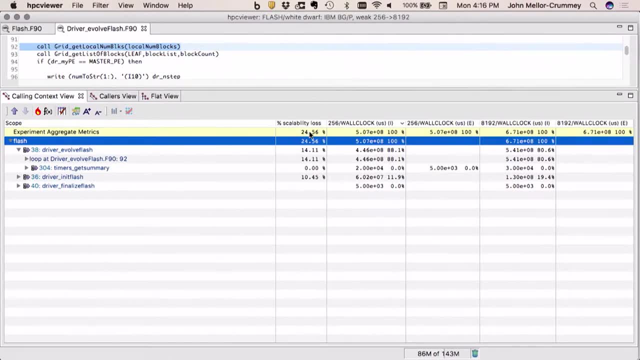 and give you sort of these seamless call stacks that'll go through the application to the GPU interface and then the call stack will continue on the GPU. So we're in the midst of doing binary analysis of GPU code. So that's kind of the high-level view. 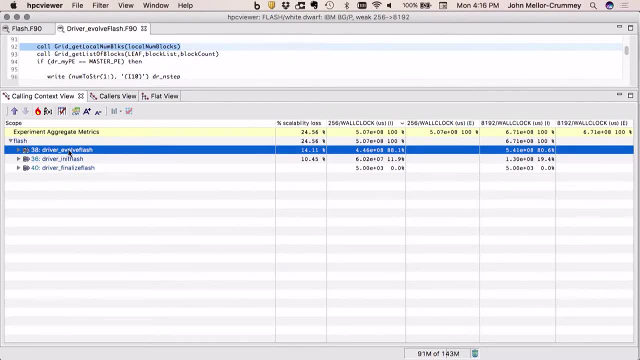 of what we're working on. So this tool set is installed on the ALCF systems And if you have copies of the slides, there's pointers to this And everything is at HPCToolkitorg. There's some help pages at ALCF as well. 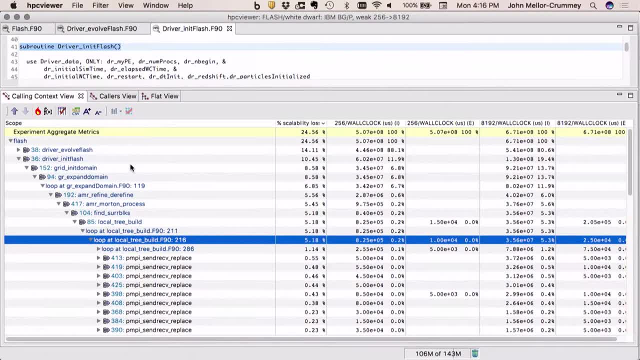 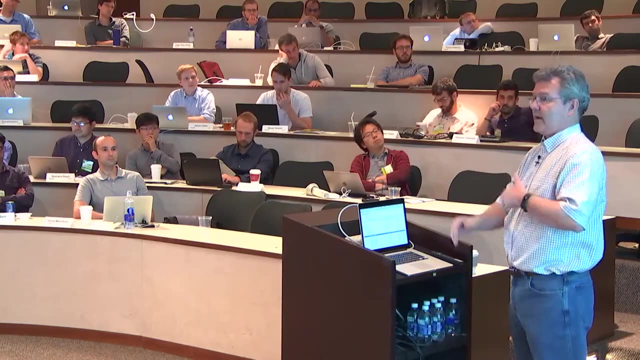 that illustrate some common scenarios And what I've doctored up for you. so there's pointers to our documentation here. What I've doctored up for you for today is: there's a GitHub repository where you can check out a copy of this algebraic multigrid benchmark. 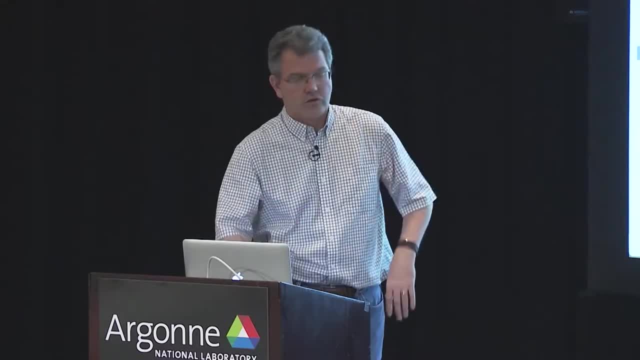 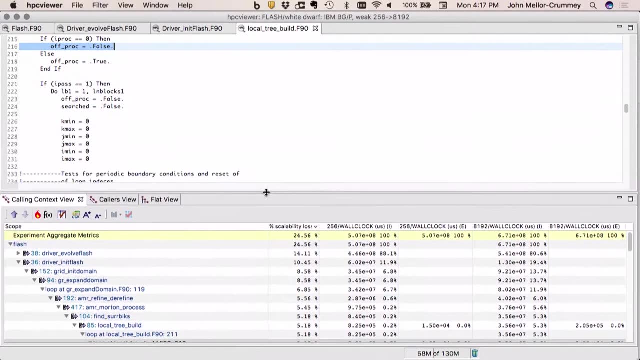 And there's a make file that will run on either Cetus or Vesta or Theta, And so I understand from Marta that the two things that we're going to be using either Cetus or Vesta or Theta. So if you say make and specify what machine you're on. 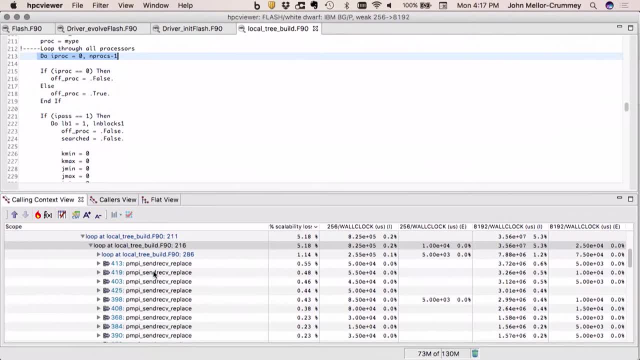 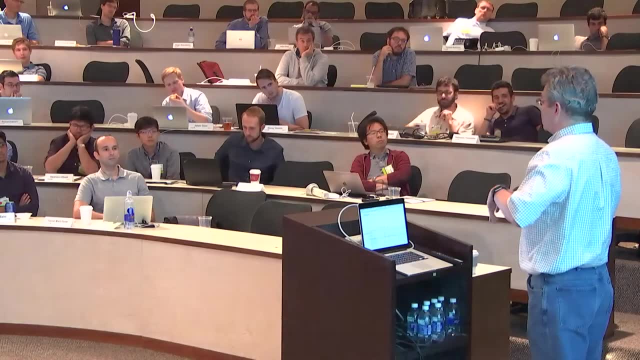 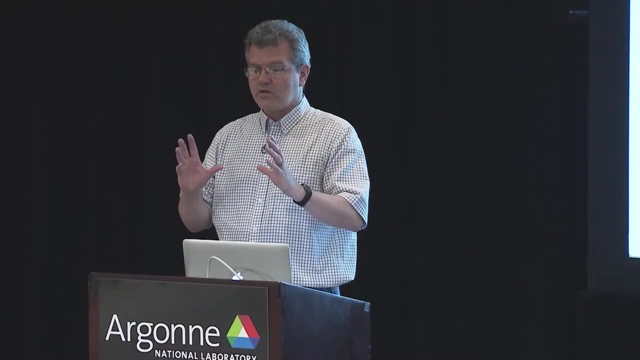 it'll do a couple of settings and then do the whole build, And then there's some launch scripts that I wrote down basically just to illustrate how one can collect data in parallel and then also analyze the measurement data in parallel, And then you can use these as fodder. 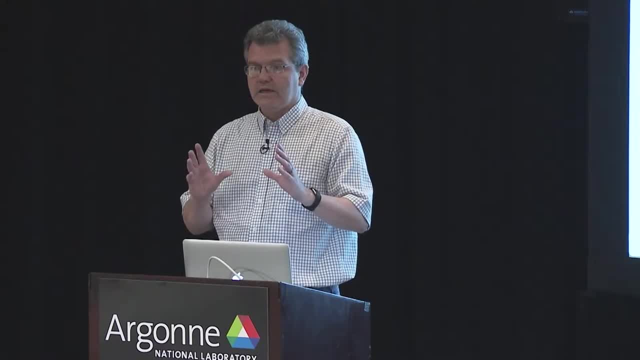 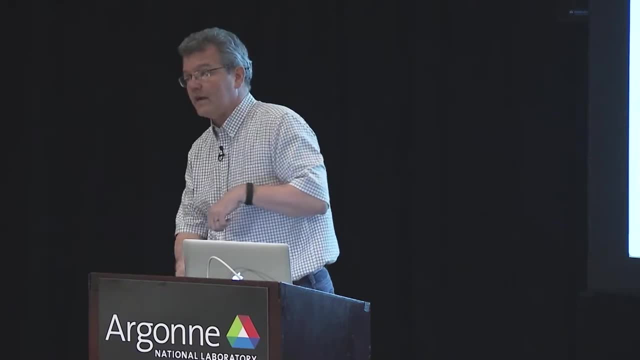 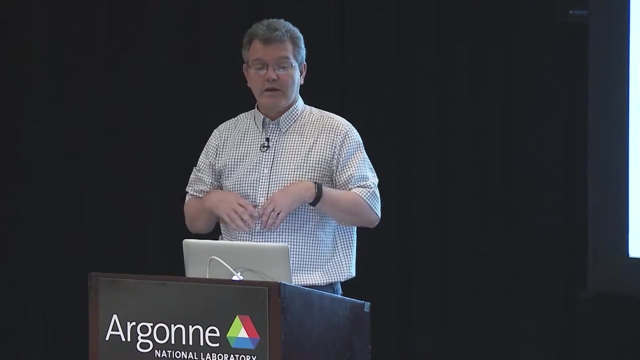 for applying the toolkit to your own application later in this session. if you don't get around to it today, You might have a chance to do it over the next couple of weeks. So I'd be happy to take any questions And then after that we can kind of dig in. 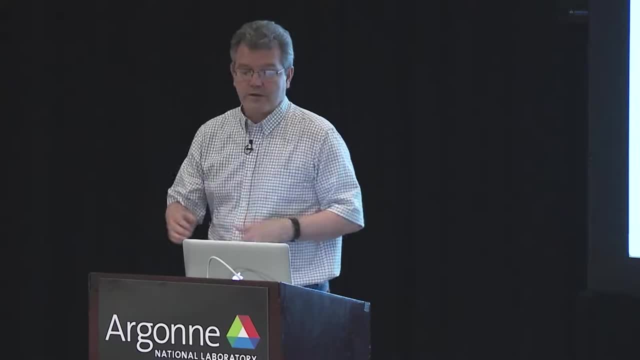 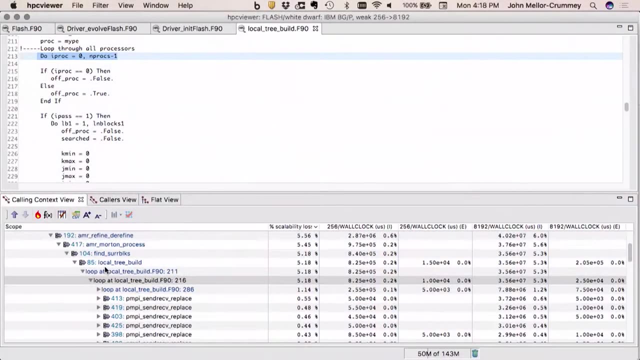 Questions. Yes, Can you measure flops and bytes? Can we measure flops and bytes? So that is a very sad story. So it turns out that the vendors used to have accurate flop counters in their hardware And then, for various reasons, 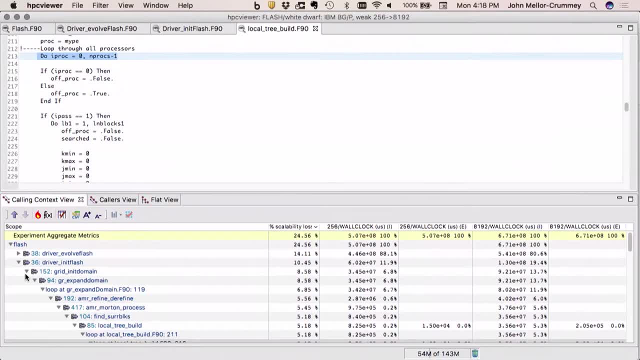 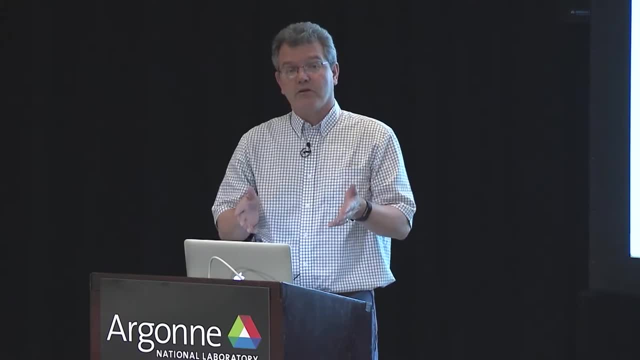 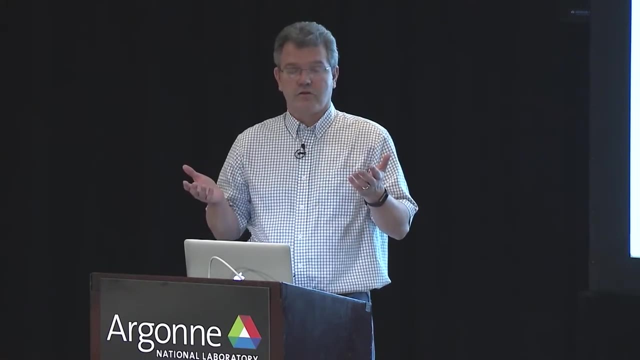 they've been getting rid of them. So on most of the architectures of interest you get very unreliable measurements. So when you issue an instruction, if it takes a cache miss or whatever, then what happens is that the hardware will reissue the instruction. 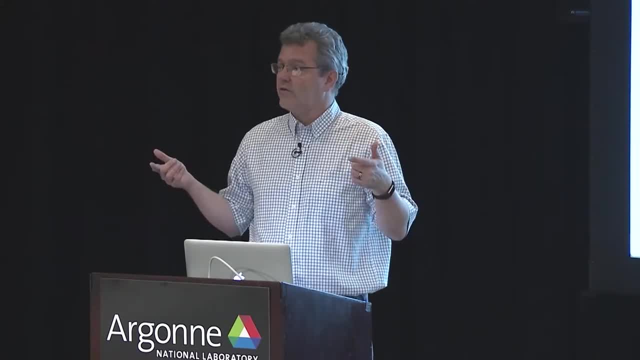 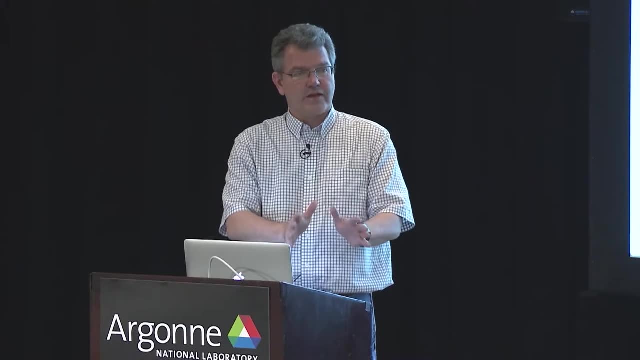 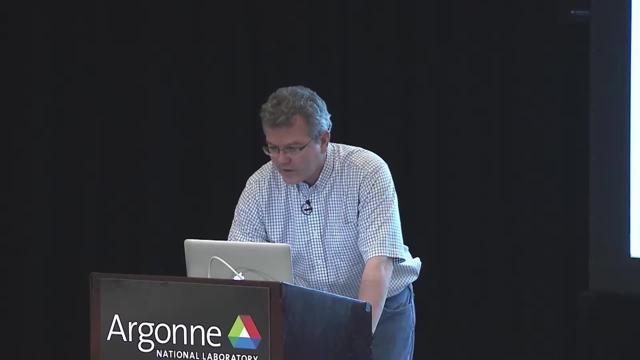 And often what gets counted are the issues, And you don't care about the issues. What you care about is actually how many instructions complete, And so if someone gives you a count that reports maybe like 20 times as much as many flops as you wrote in your program. 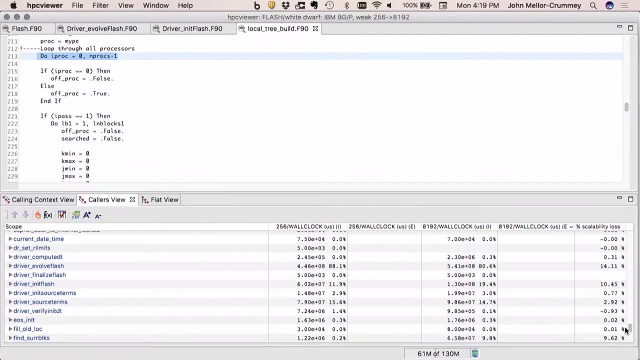 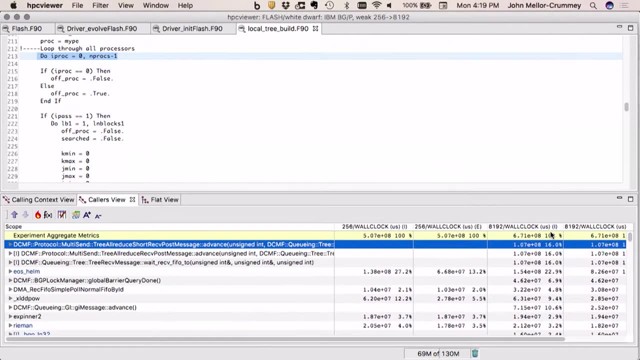 that's not very useful. So the status of flop counts is not so good, But we have a plan. We can actually measure graduated instructions very well, which means we can measure that instructions are completing And if we tie that together with binary analysis. 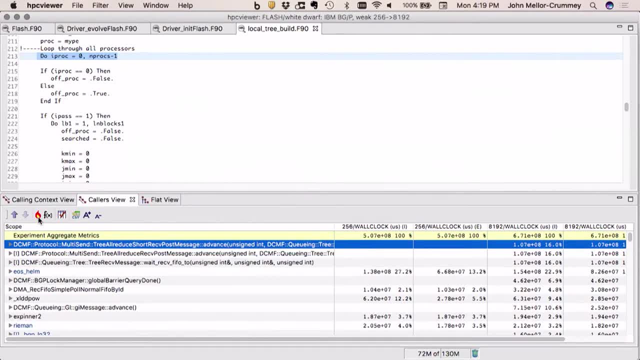 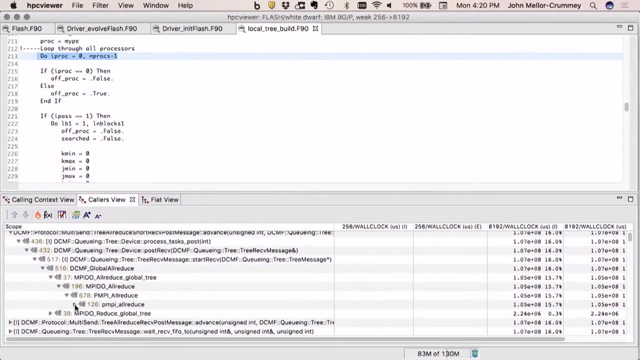 we can look at this instruction completed or we sample this instruction completing. so many times Was that a flop or not? But that's sort of a twinkle in our eye at the moment. We did this a long time ago for the alpha. 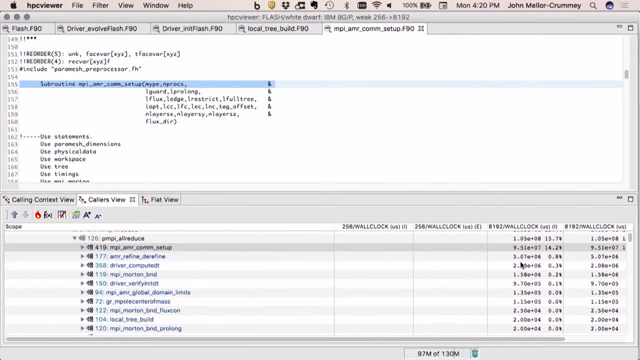 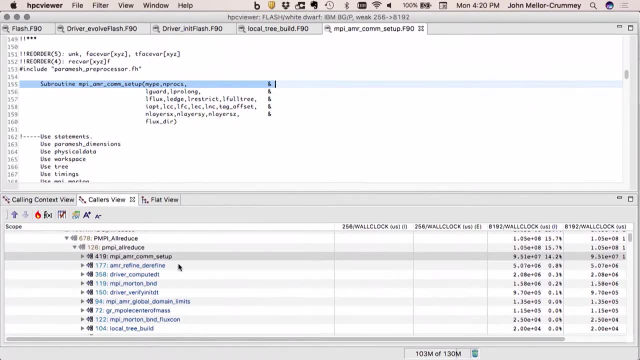 but it turns out that now that the counters have gotten worse, we have to go like back to this technique. Now, in terms of data movement, we can watch things move in, like with cache misses. we can watch it move in the upper levels of the memory hierarchy. 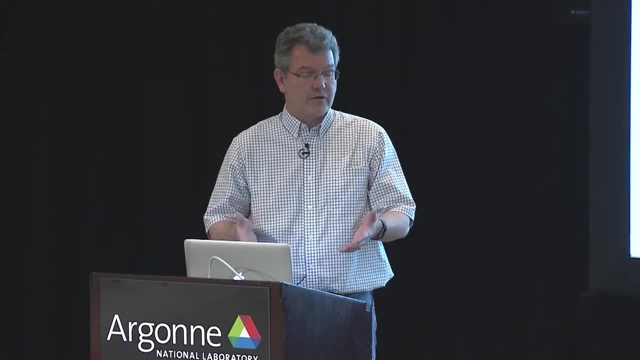 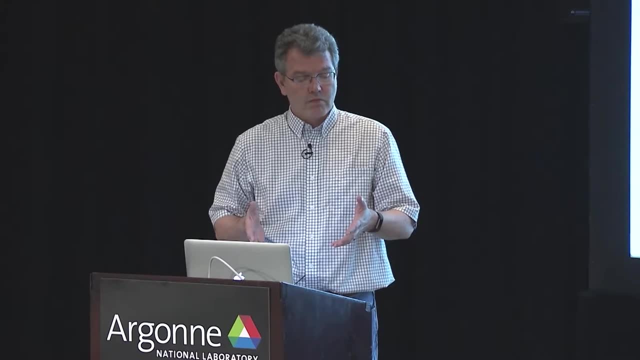 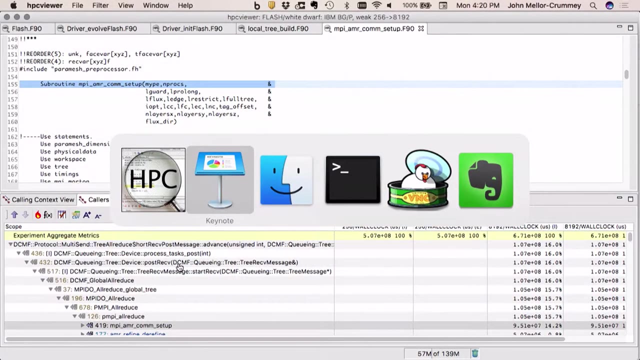 but we can't- really we can't- sample, as things are moving from the memory interface out. Now there are some architectures will tell you that you're getting your data from memory. There's the load latency facility on the Intel architectures and there's something called instruction-based sampling. 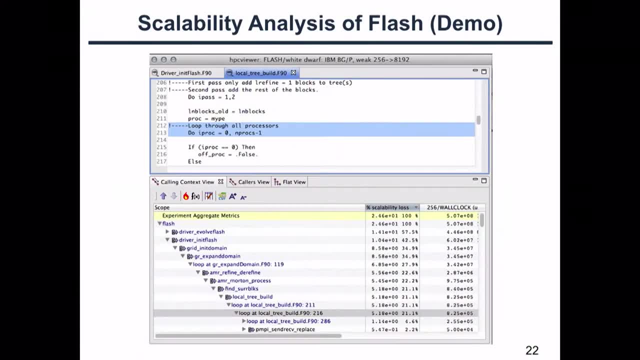 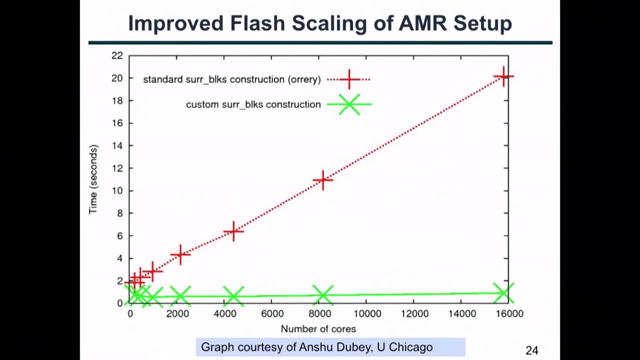 on the AMD architectures And so you can find out like where you got your data from and what latency. but you can't count all this stuff out at the edges because the counters are like nowhere near the cores and it's like counting shared stuff. 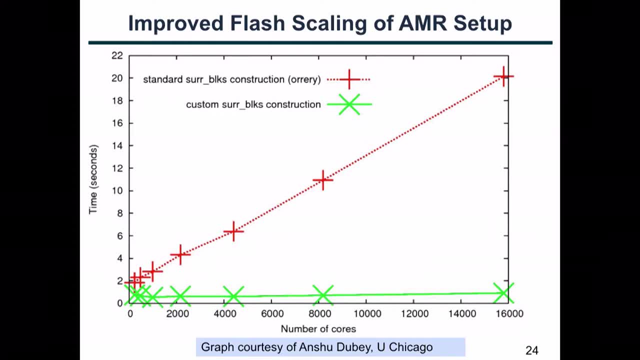 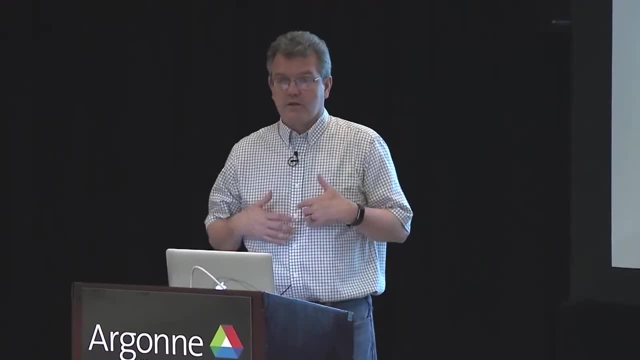 and so it's hard. Now on the blue gene, we can count L2 cache misses, but we're counting aggregate across all of the cores, and so we can't say this is my millionth miss. What we can say is like: a million misses have occurred across all the cores. why don't we interrupt everybody and ask, like, where you are? And so, instead of having a finger pointing at you, saying, like this is a spot that, like, is generating misses in your program, 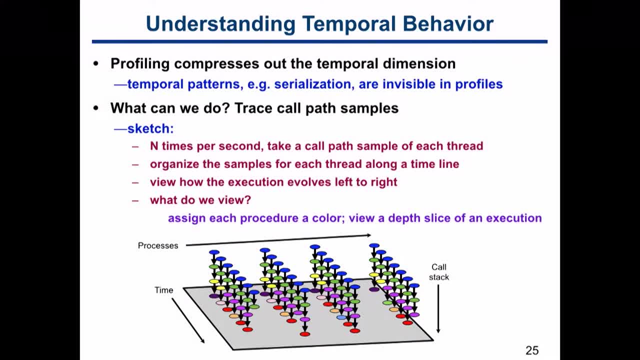 instead, what you end up with is like likely suspects and, like you know, is it a likely suspect or just an innocent bystander? Well, if the counts keep accumulating, probably it has something to do with it, but it could just be an innocent bystander. 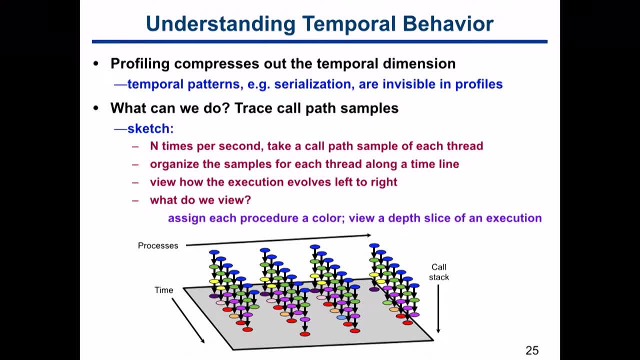 So we don't actually have this tight correlation between memory activity and flop activity and your code, so you have to be a little bit crafty about things that we measured to gain some insight. unfortunately, It's like not our fault, okay. 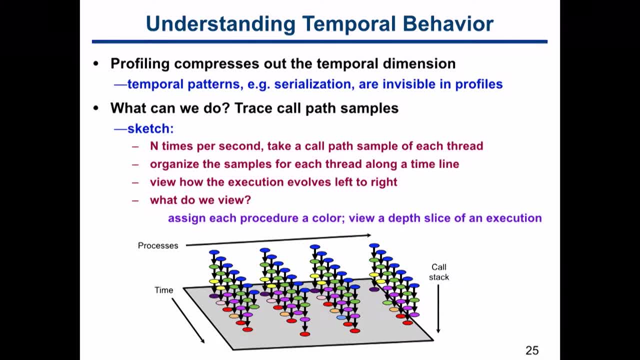 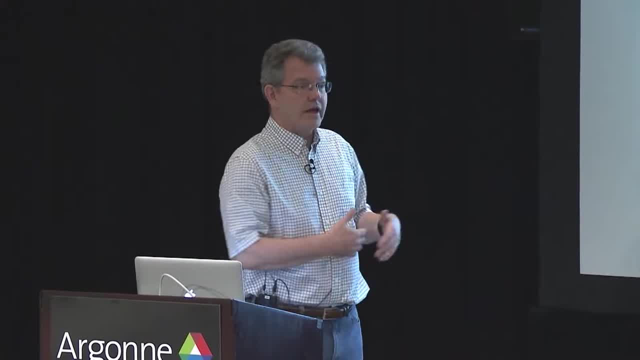 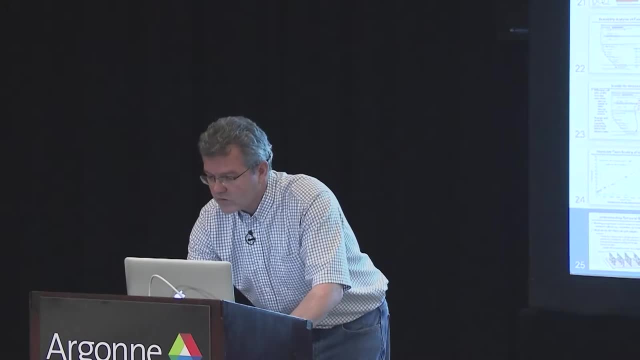 Blame the architects. Other questions: Yes, So is this meant to replace, like for GPUs, like NVIDIA's profiler? Yeah, so it turns out that like the NVIDIA's visual profiler, so what they're able to do? 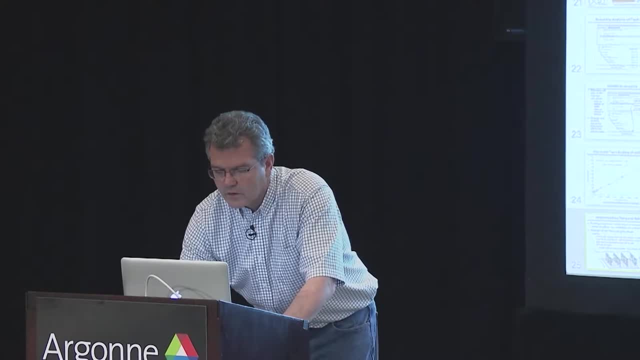 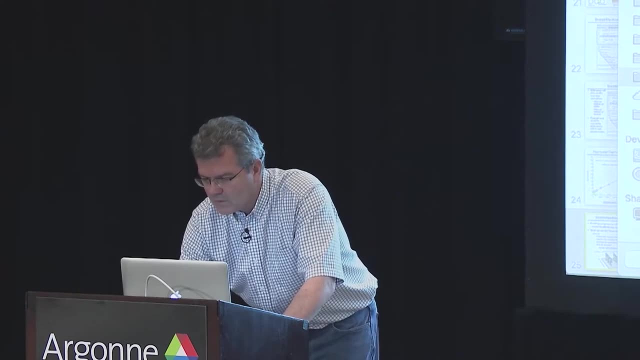 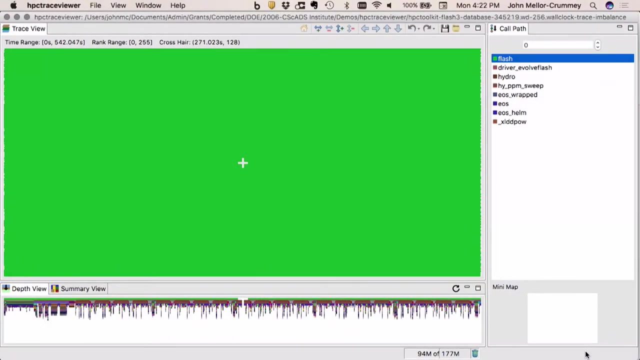 with that. now, based on the support for sampling that they put in their GPU, you can actually attribute stall latency, like you know, whether it's like a stall for waiting for data to come from the GPU memory or waiting for the data to come from cache. 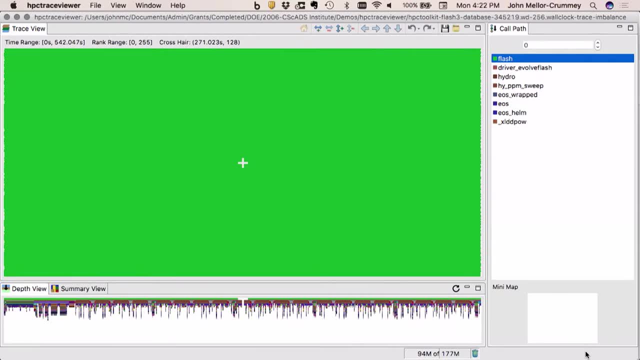 or something like that, or you're waiting for another instruction to complete. You can attribute these stalls to instructions in the program, So we are going to be able to do the same thing Now. the difference is that, like NVIDIA, most of their 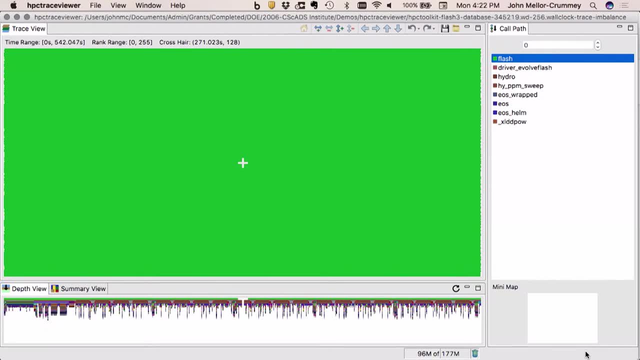 tools are like largely timeline-based and they collect timelines for like a GPU. So think about how you're going to measure something that's like running on like thousands of nodes with thousands of GPUs And so. 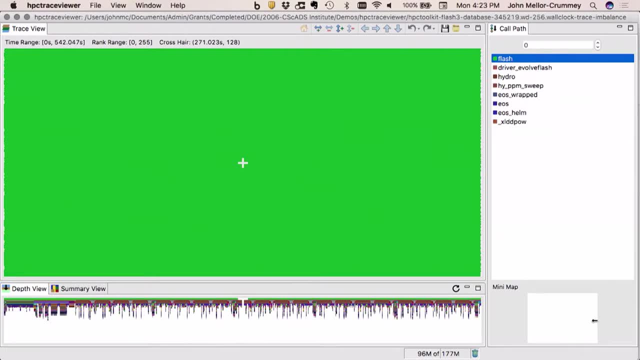 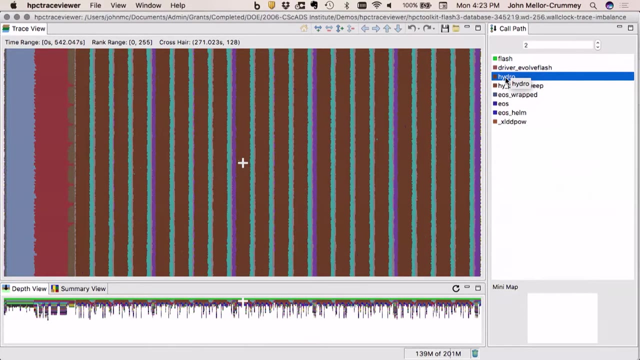 our strategy for measuring these timelines and rendering them at multiple levels of scale. we've applied this to GPUs already, and we're now looking to do this with the sampling-based hardware on the GPUs as well, So I think that they can help you if. 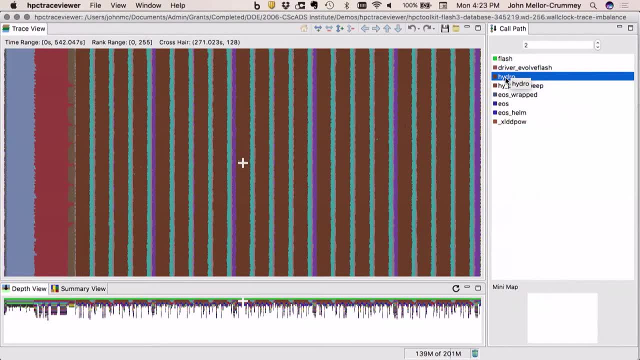 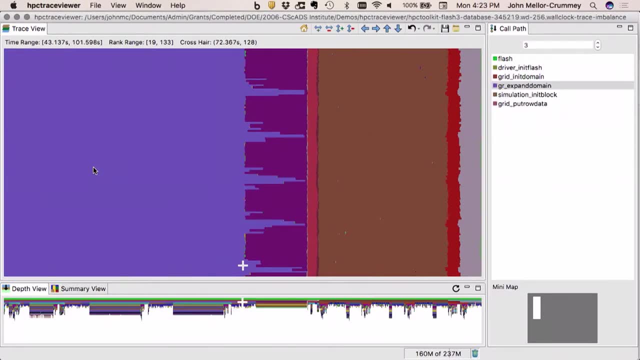 what you want to know is like: exactly how am I spending my time in some kernel F? But what you actually have to ask is: do I really care about the performance of kernel F, Or are all my processes active, Or are my? 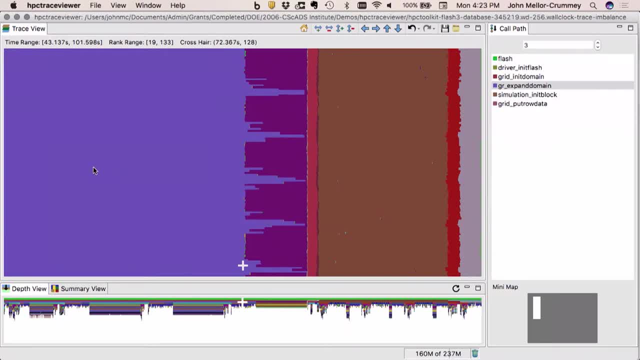 threads active, And so you really need to know, like, who's doing what and who's synchronizing and waiting for whom, And so, even if you're computing with really high performance, if you're never in this routine, it doesn't matter, right, And so 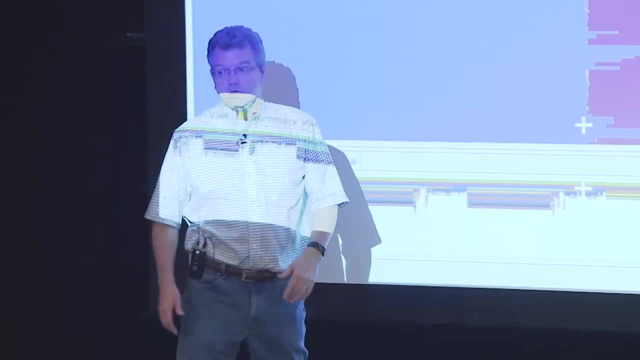 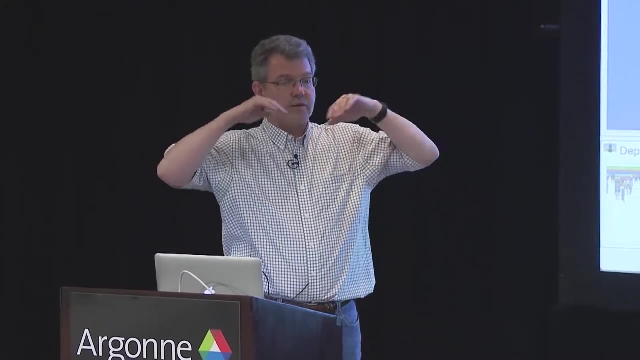 I think that you have to take this top-down perspective to ask: are all my nodes computing? Are all my threads computing? And like issuing work to the GPUs, is the GPU computing effectively? But we only care if the GPU is computing effectively, if it's like mostly busy. 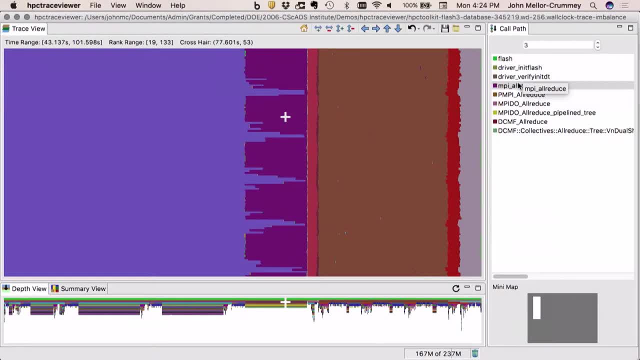 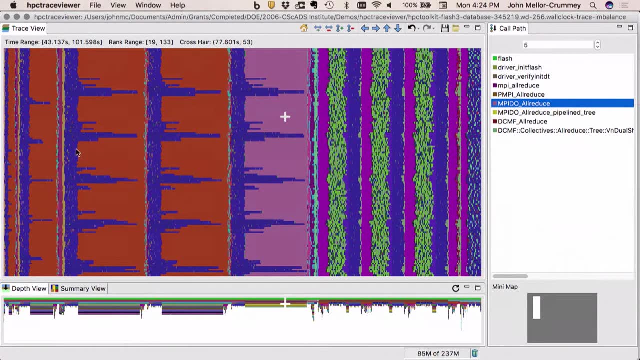 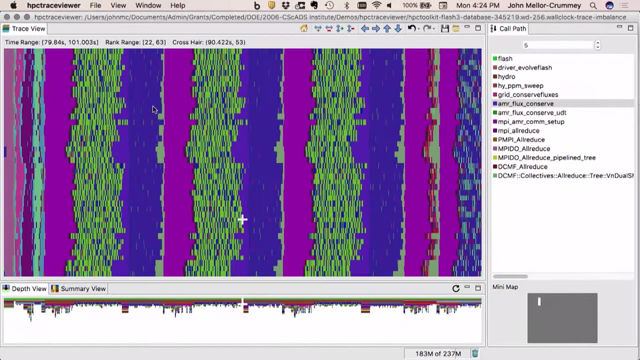 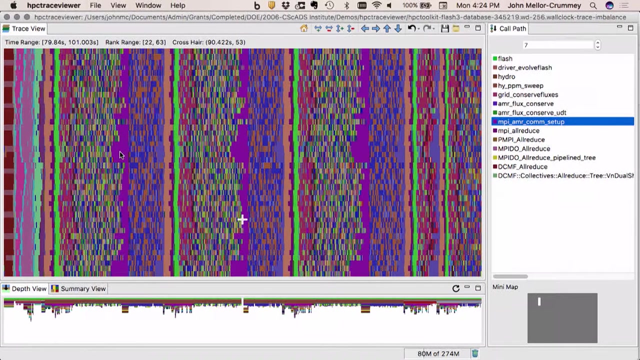 Right, Okay, Other questions. Yes, Besides the pre-visual output, what do you think AHP SQL kit does better than V2 and other software? Because a lot of the functions are pretty similar. Yeah, so it turns out that they've been copying us for a while. 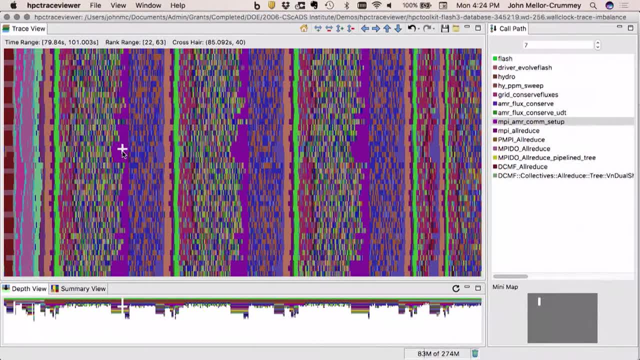 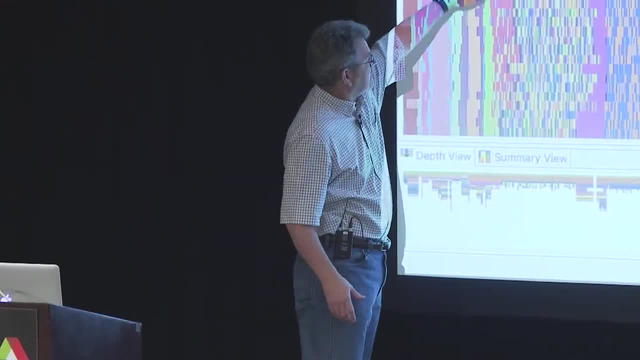 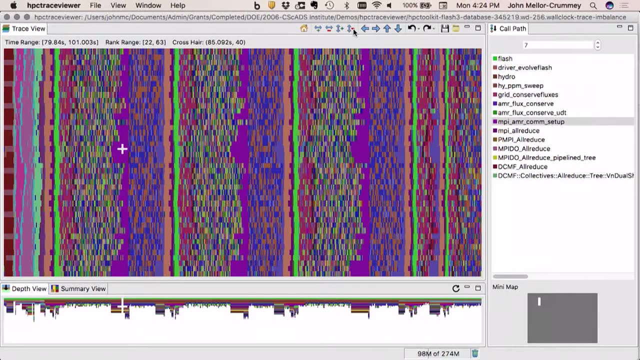 So this whole sort of three views, this top-down, bottom-up, that was ours. first The timelines, for, like the large-scale timelines that was, we're collecting these using sampling. Intel's VTune is collecting these using tracing. 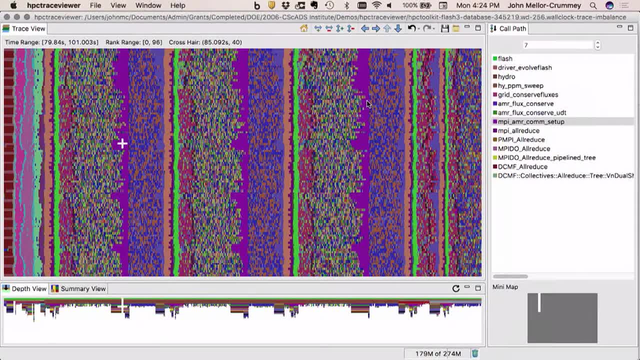 Try running it on a big program or on a long-running program. I can show you data from an application running on 8,000 cores for 20 minutes on my laptop. I dare you to try that with one of the Intel tools, And the same thing is true with. 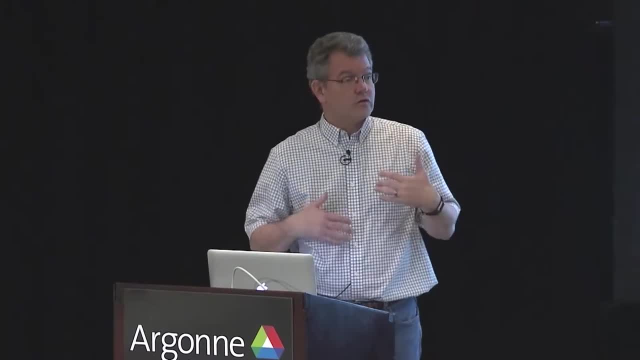 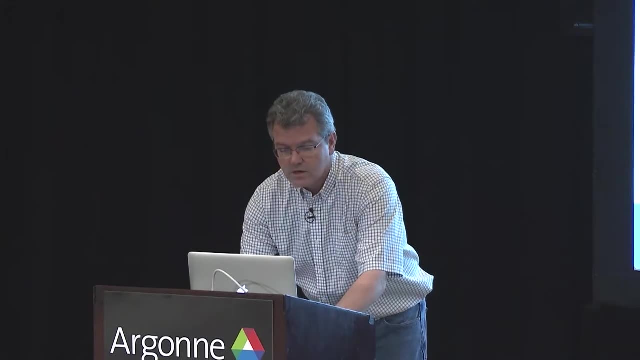 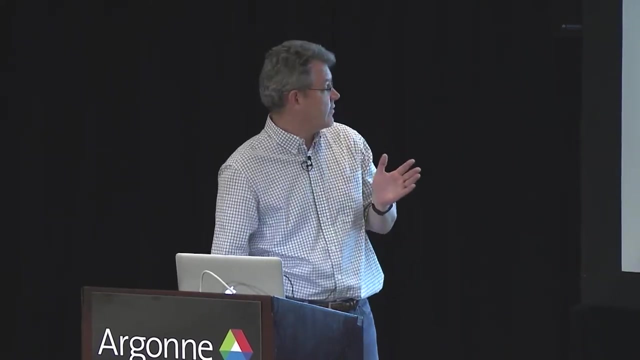 NVIDIA's tools. They are collecting these large-scale traces, And so when you're tracing, like every kernel launch and every function entry and exit, you're accumulating data at gigabytes per second. Okay, We don't do that, And so 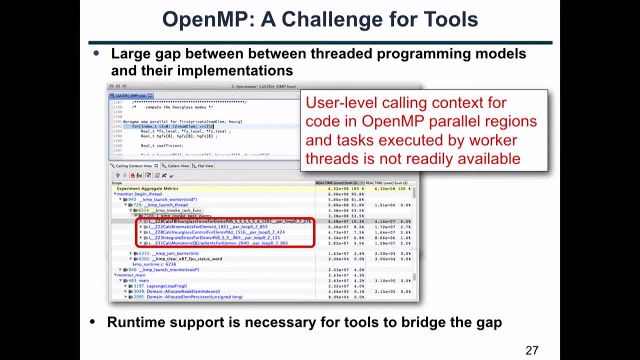 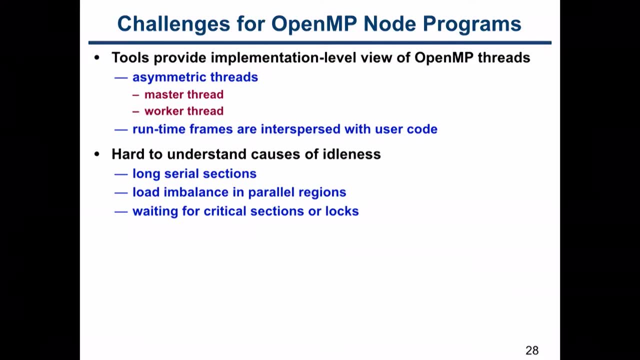 what we've been trying to do is to push this sampling-based measurement approach, where we can gain insight, like using this scalability analysis, while also collecting just a modest amount of measurement data. Okay, So I think that that's really the thing that we've been focused on. 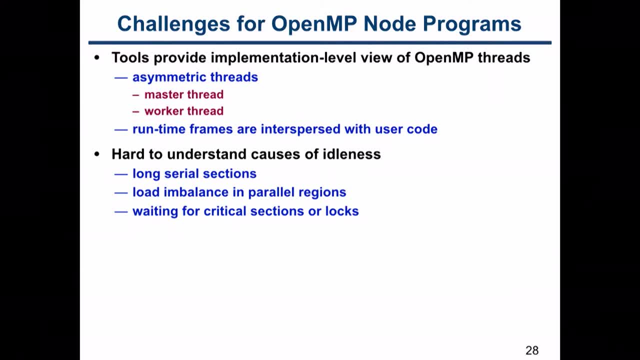 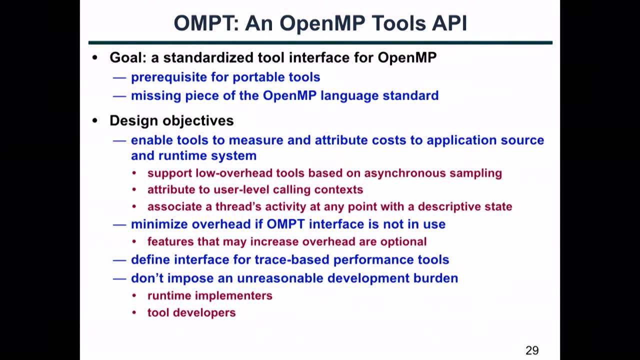 And so we've been pretty successful. We won a best paper award in PLDI. There was a best paper award that one of my students won in supercomputing back in 2015.. So the things that we're doing, they're innovative and people are. 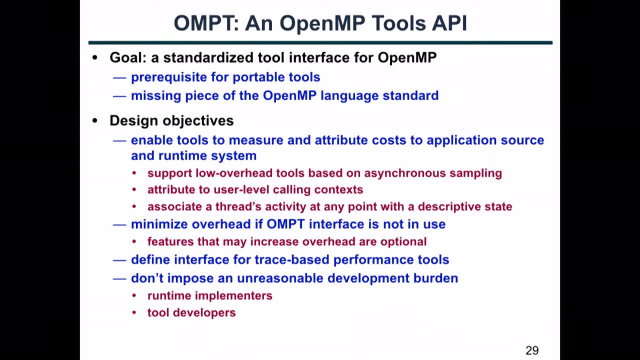 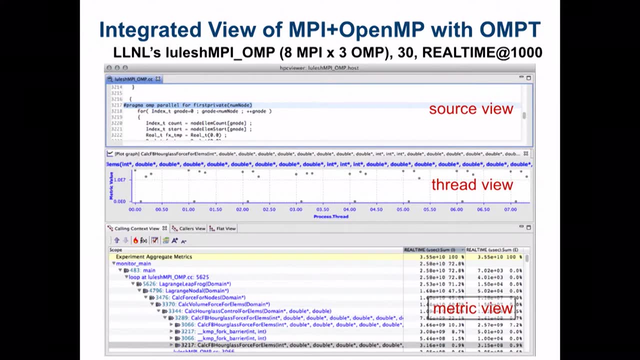 copying them. So if they look similar, you have to look at where they came from. Okay, Yes, So earlier today we heard that we should put things like profiling in the code right from scratch rather than adding that later on. So now that looks like. 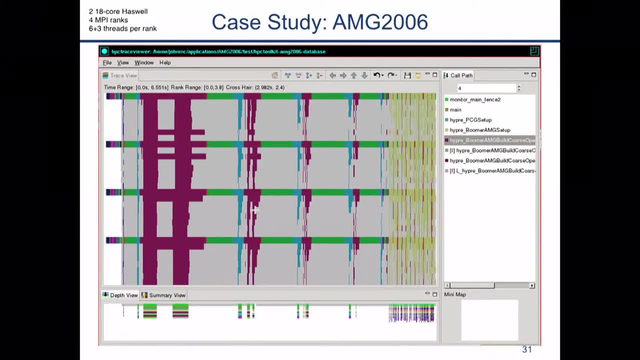 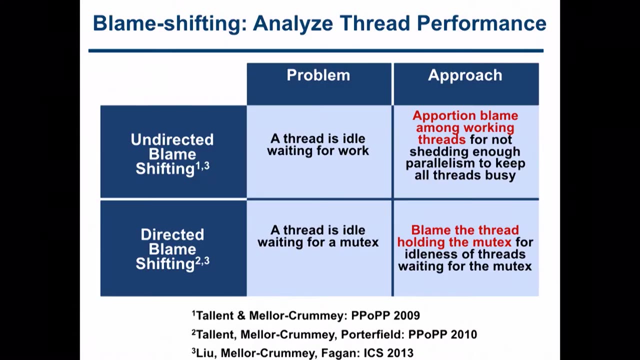 we should not be concerned with profiling at all, because it can be done on the binary level. Yes, Okay, So you should say that there's a war between the folks who believe in instrumentation and the folks that believe in measurement with sampling, And it depends what you want to measure. 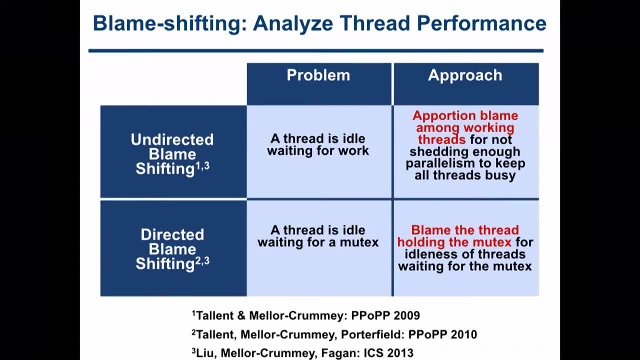 So if you want to put in instrumentation, so, for instance, we could automatically add instrumentation that would count the amount of bytes moved by MPI, Okay, Just by adding this function wrapping. There's also this darshan layer from Argon that measures IO, And so for measuring. 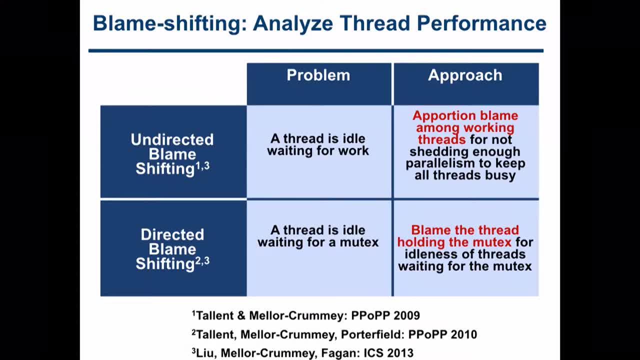 semantic information like data moved or whatnot. having an instrumentation layer in there makes sense. But to physically have some routine invoked every time you exit or enter a function or exit or enter a loop, you will distort your program so fast if you're measuring things like that. 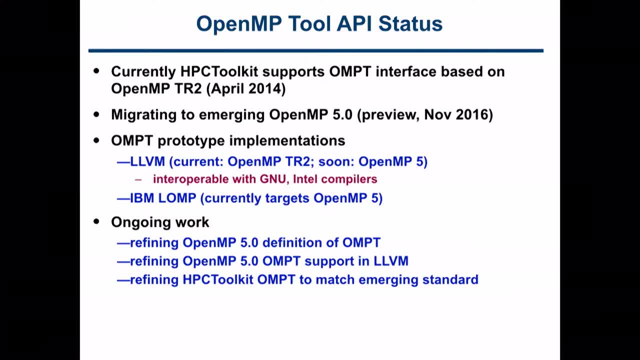 Now, if what you want to do is measure your flow phase and measure your transport phase and you have these coarse-grain timers around the outside, have at it. That's not going to get in our way and it's going to give you some sort of coarse-grain. 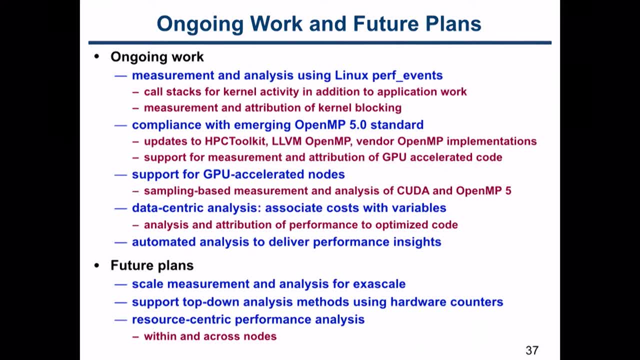 information about what's important, But if you want to figure out how you're going to make it faster, knowing that you spend 70% in this and 30% in that isn't going to help you fix it. Other questions, Yes. 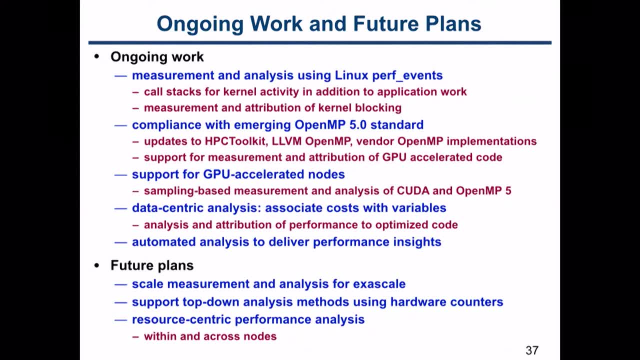 Can you say that the overhead of this is low enough that I could just use HPC Toolkit on all my runs and just feed home for that, in case I ever want to look back and see what actually happened to some production stuff? So I guess I would not. 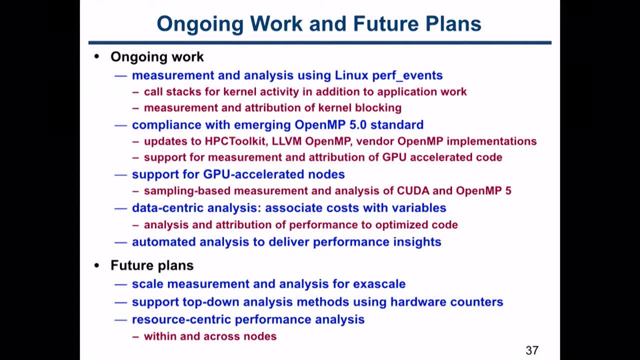 advocate using it for all runs, But Livermore is actually looking at doing this kind of thing, So what they would like to do is to have an API that would allow them to kind of turn it on and turn it off and mostly just leave it in the background and 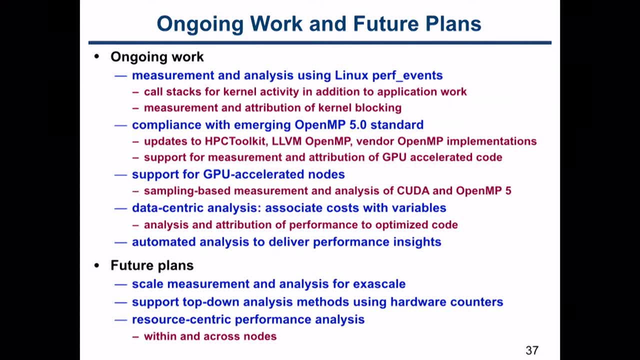 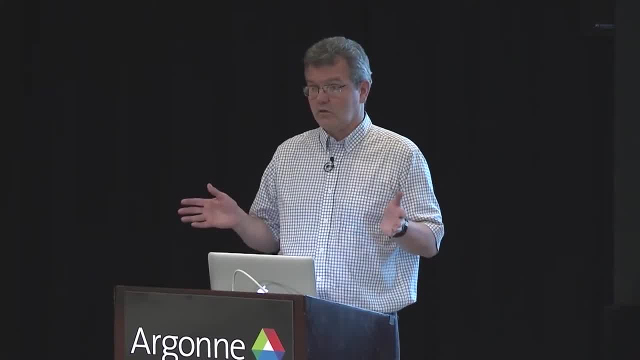 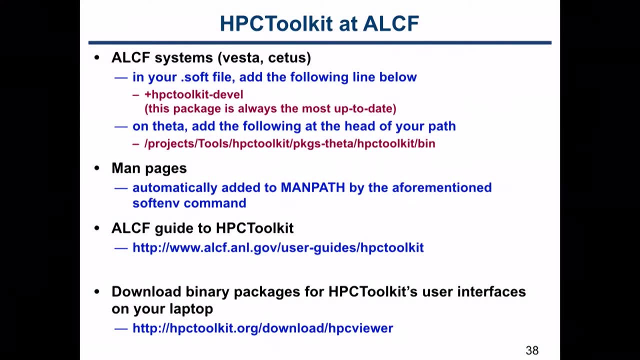 basically collect performance analysis everywhere, all the time and with a low enough sampling frequency so that it's basically unobservable, And so I think that that's ultimately our goal, and right now it's not as automatic as you would like, because 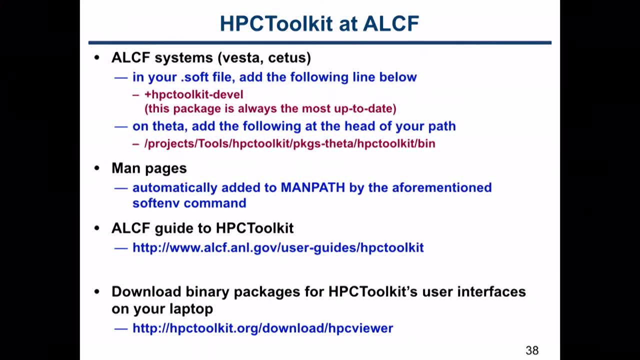 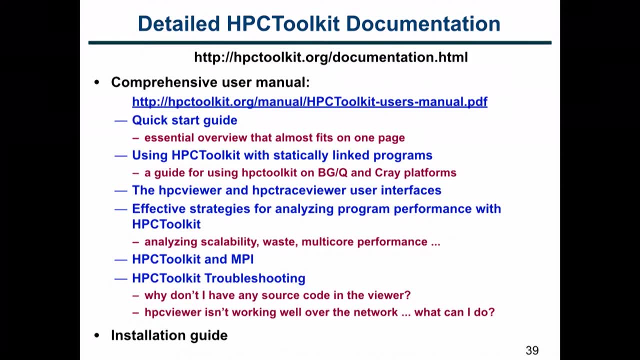 this started out as a research tool, and so we say: hey, you have 400 hardware counters in your processor, Pick which ones you want to measure. Well, that's not the best approach for an application scientist, right? What we should say is: well. 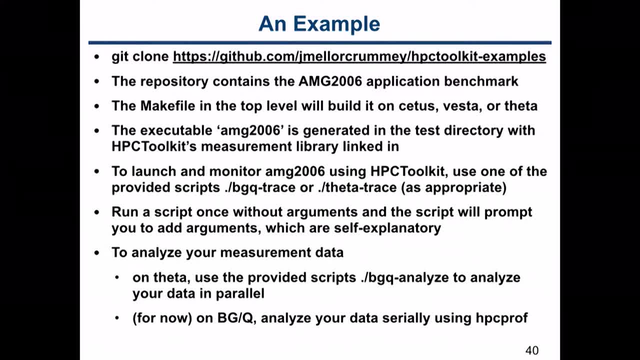 so if you want to study the memory hierarchy, then maybe you should measure the interplay of these particular counters, and so that's something that a vendor like Intel does better than us. They're working on support for these top-down models. That's something that's.